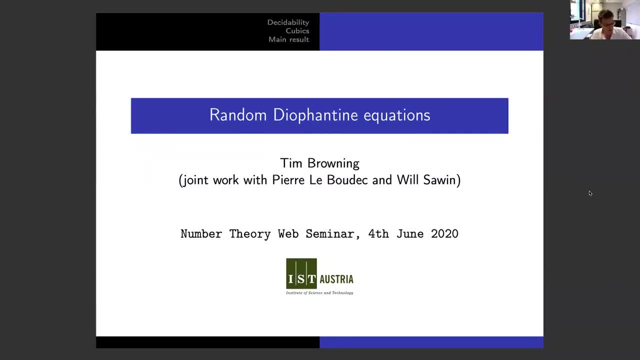 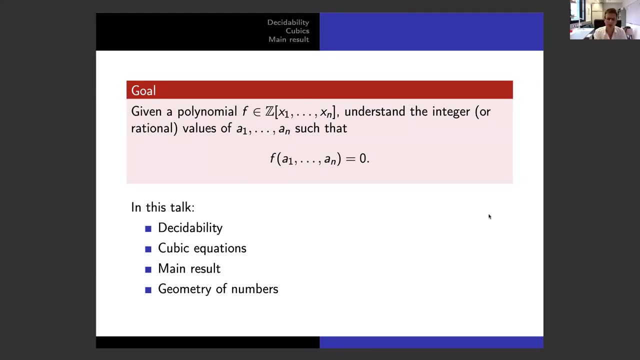 And I think we've now, as you can see on the archive, we've put this to rest. So this talk is all about Diophantine equations. So these are just polynomial equations with integers, These are integer coefficients, and we want to understand when we have integer or possibly rational solutions to these equations. 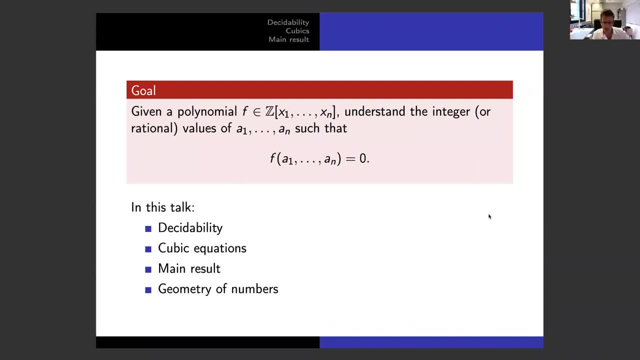 So I'm going to keep this talk fairly colloquial, I think. to keep the analytic number theorists happy, I will certainly introduce some iterated logarithms. I might change the order of summation at some point, but the rest will be at a very sort of gentle pace. 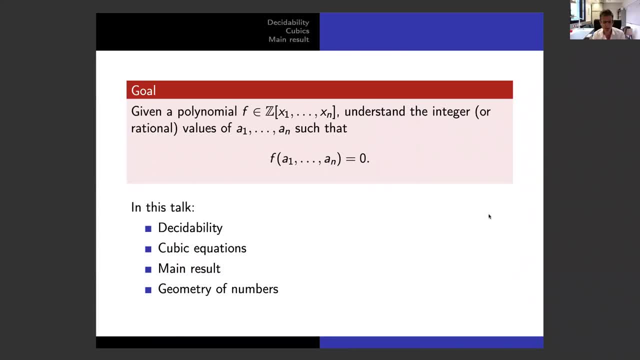 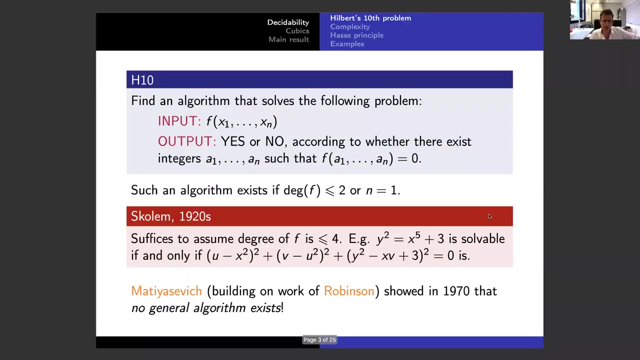 I want to start by talking a little bit about the decidability problem for this question. I will focus on cubic equations for a little bit and then I'll talk about the main result and how it's proved using the geometry of numbers. So the kind of famous result or question here goes back to Hilbert and his famous address at the turn of the previous century. 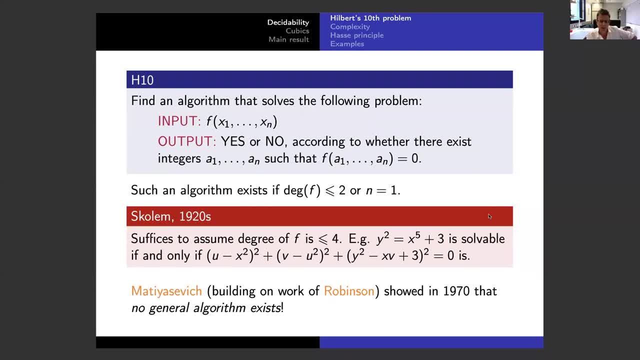 Previous but last century. And he asks for an algorithm about whether you can, given any Diophantine or any polynomial with integer coefficients, can you decide whether or not there's an integer solution. So this is known when the number of variables is very small, so for polynomials in one variable, and it's also known if the degree is at most two. 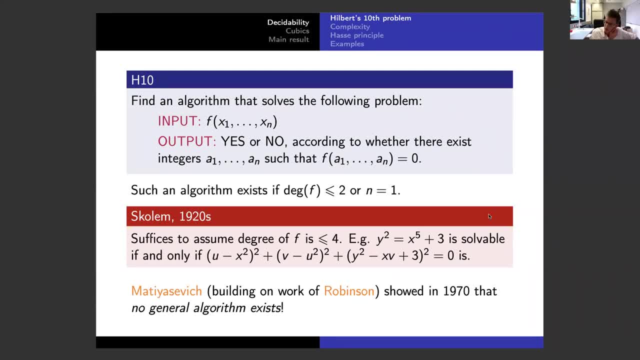 In fact it was a nice observation of Scolom- using the non-negative, non-negativity of the zero And in fact it suffices to always assume that you've got polynomials of degree, at most four. That's an example there involving the Model curve. 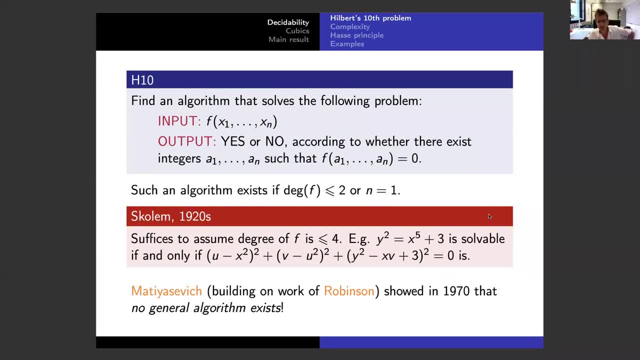 But we now know this dream of Hilbert can't be attained. There's no general algorithm for deciding whether or not any given Diophantine equation has a solution, And, in the absence of that, we're left with finding perhaps classes of Diophantine equations that have no answer, and not something that we could quite simply define. 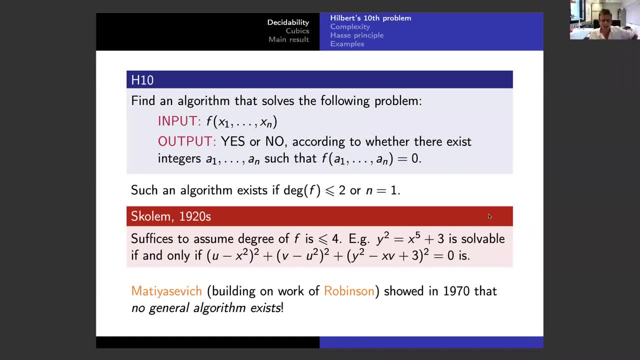 So, to summarize, here's the question that we need to find: What does this mean? What does this mean? Well, this means that we've got sub даже, sub even and sub even. We're missing the root of the answer. 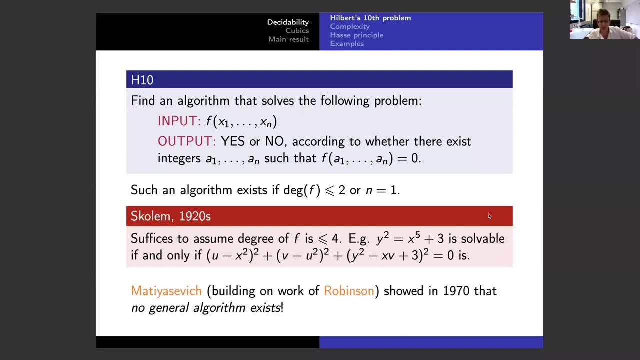 So the answer is the right answer. We need to find the root of the answer. They're both pretty symmetric, So we've got sub, even on the right side of the equation, equations for which we can exhibit algorithms. But I want to point out that 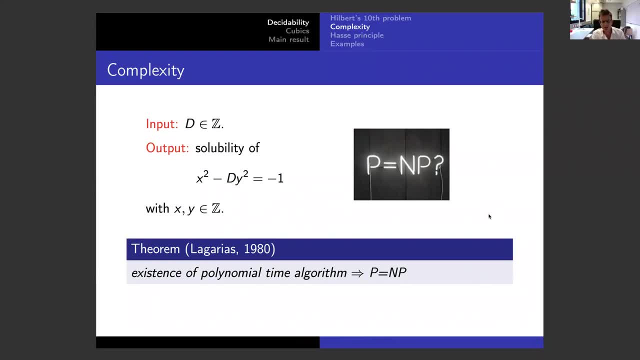 even in the case of very simple quadratic equations. it's just a quadratic equation in two variables. there remains much that's unknown. So there's a nice paper of Jeff Ligarius from the 80s who discussed the algorithm for deciding the solubility of the negative Pele equation. So here you. 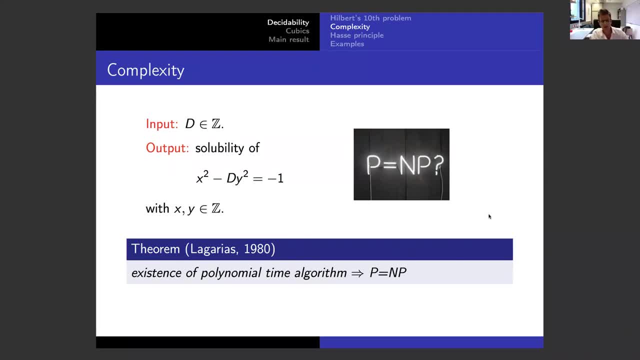 you just look at the continued fraction of D and the equation is soluble if, and only if, the period of the continued fraction expansion is odd, And in fact Ligarius proved that this is an NP algorithm. so if you manage to come up with a polynomial time algorithm, 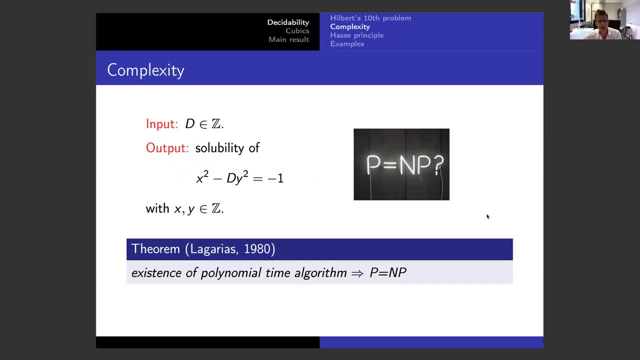 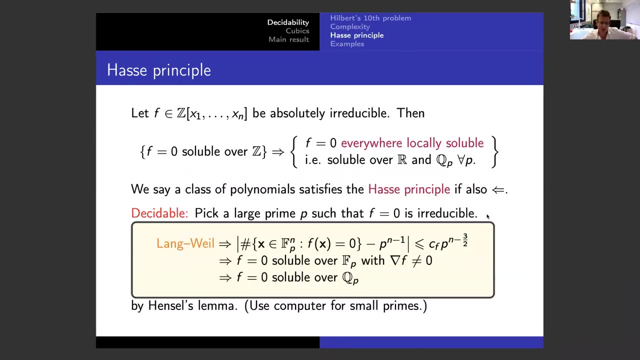 particular, solve this thorny issue of p is equal to np. I think it's unknown whether or not this is in np complete, but I just wanted to illustrate that even in the case of degree two equations, there's much that's unknown, So the kind of main test for solubility that's going to motivate this. 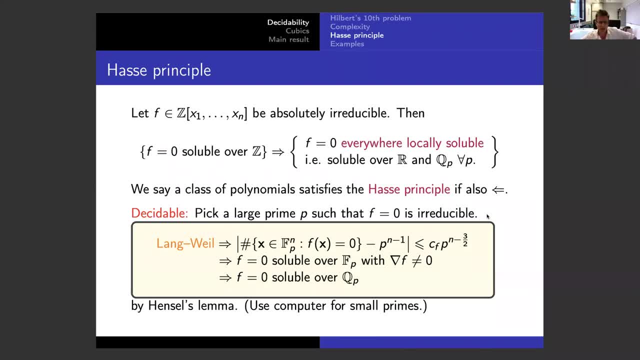 talk comes from the most obvious necessary condition for solubility, namely it should be soluble over all of the completions of q, so it should be soluble over the reals and over all of the piatics, or, if you like, at modulo, every prime power. there should be a solution. So we say that. 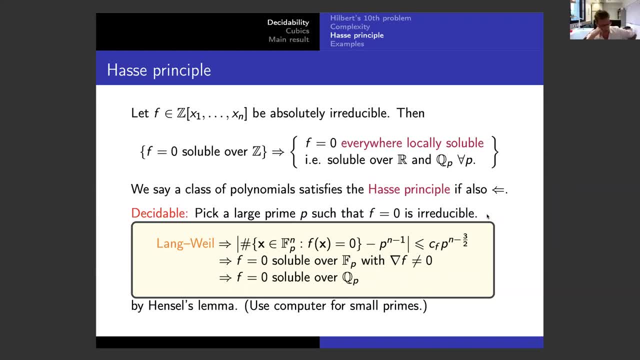 a class of polynomials satisfies the Hasse principle if this necessary condition is also sufficient. and this is a nice thing to have when you know that a class of polynomials satisfies the Hasse principle, because this is in fact a decidable problem. So let me discuss it briefly. in the case of 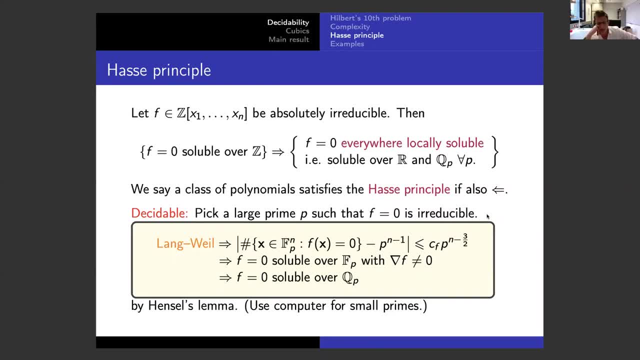 decidability over the piatics. So for this you just want to pick a large prime p, such that this polynomial remains irreducible when you reduce it. modulo p, Then by invoking the Langvay estimates, which is a sort of generalization of the. the resolution of the. 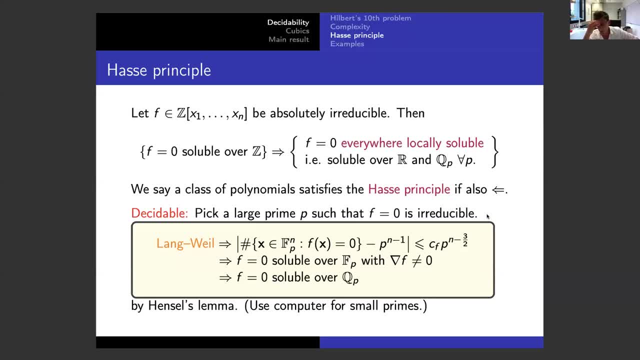 Riemann hypothesis for curves. this tells you that the number of fp points on your hypersurface, or number of fp solutions to this equation, can be approximated by p to the n minus one plus an error term, which is smaller. So, in particular, again, if p is large enough, that's. 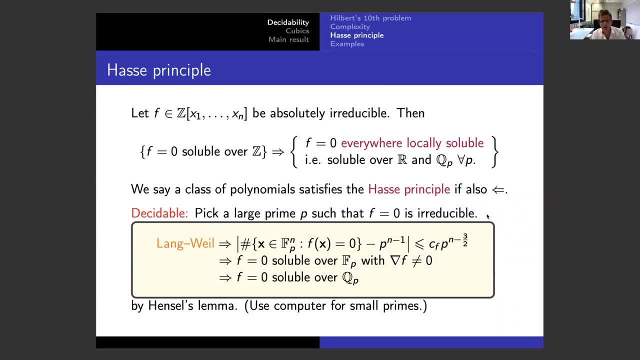 enough to guarantee that there's a solution over this finite field in which the partial derivatives of your polynomial don't all vanish. And now you appeal to Hensel's lemma- which really just goes back to Isaac Newton, I think, and that allows you to lift these fp solutions to get genuine solutions over qp. 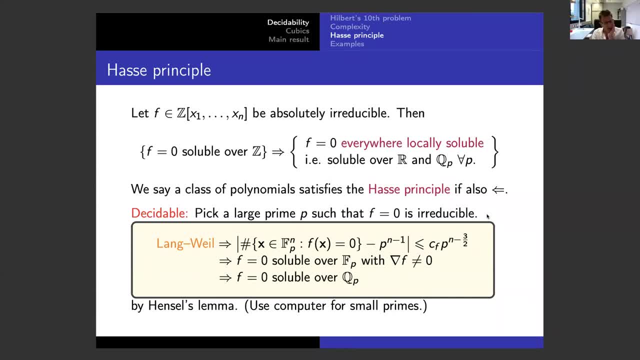 Okay, so large primes, you automatically get p-addict solubility. and then for the finitely many- and in fact we're going to talk about this in a bit- So large primes, you automatically get p-addict solubility. and then for the finitely many- and in fact we're going to talk about this in a bit- 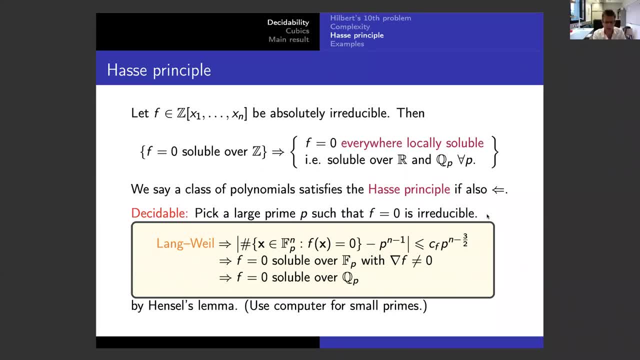 So large primes, you automatically get p-addict solubility. and then for the finitely many- and in fact we're going to talk about this in a bit- So large primes, you automatically get p-addict solubility. and then for the finitely many- and in fact we're going to talk about this in a bit- 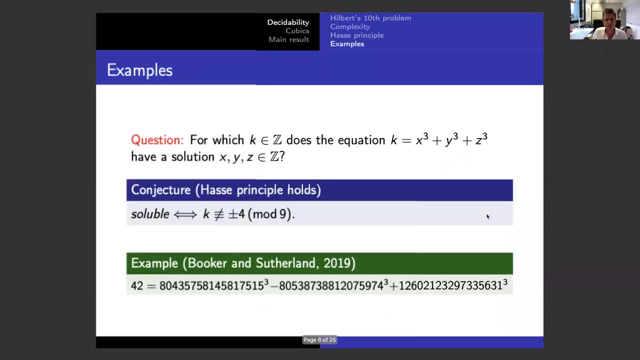 small primes and just use a computer, do it by hand. so in principle this has a principle, is decidable. Nonetheless, it's very. they still present, though. demon equations still present lots of challenges, like quadratic equations, as I've discussed, and cubic equations. so this is a question I like a lot: which integers are representable as a sum of three. 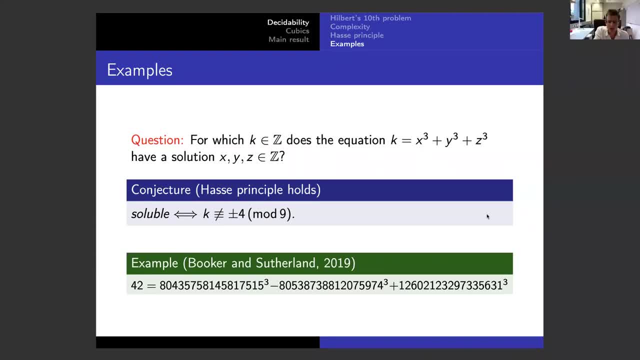 cubes. so the local condition here, the local test, is that your integer shouldn't be plus or minus 4 mod 9, and we saw a beautiful talk by Drew Sutherland in this series a few a few weeks ago. it's a sort of very beguiling. 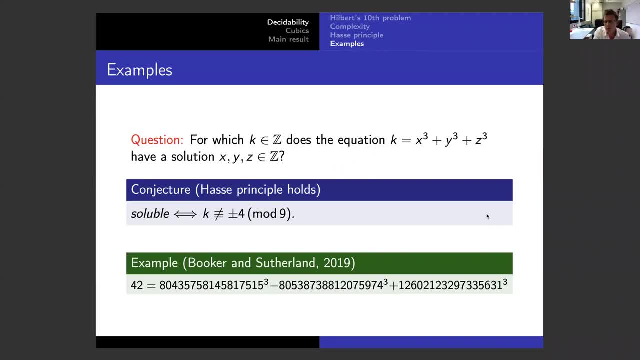 problem because for some K you get very small solutions. so if you take K to be 3, it's not very hard to work out what the smallest solution is in that case. but if you take other values of K, such as the number 42, it took an enormous. 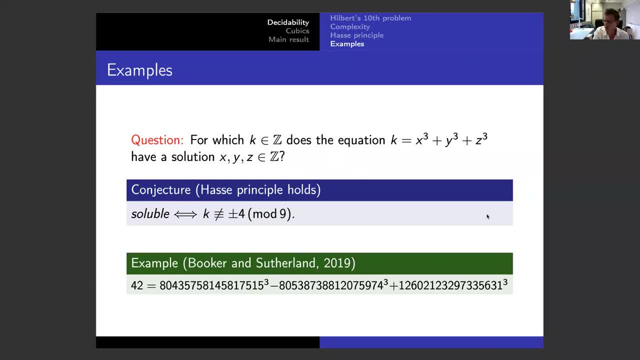 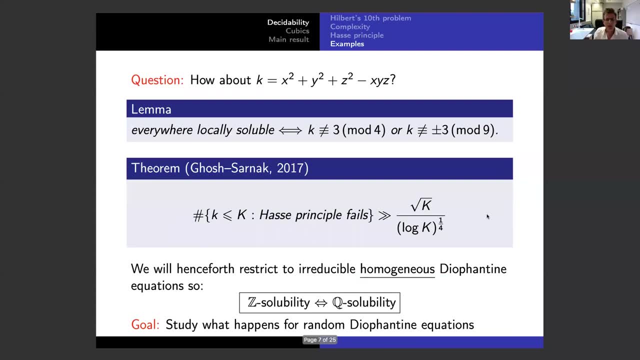 amount of ingenuity and computer power to actually write down the smallest solution. one might ask about other cubic polynomial representing integers, and in fact you get a different story sometimes. so here we're asking about representations of integers as sum of three squares minus the product of the variables X, Y, Z. again the local test. it's quite easy to work. 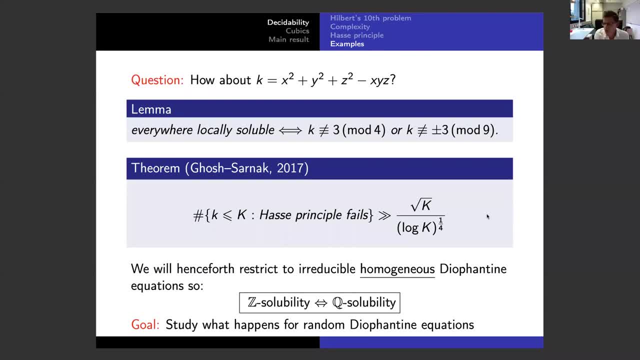 out that provided K is not 3 mod 4 and not plus or minus 3 mod 9, that's enough to guarantee solubility over all of the piatics, but nonetheless this is not necessarily enough to guarantee that there are solutions over the integers. and there's very nice paper. 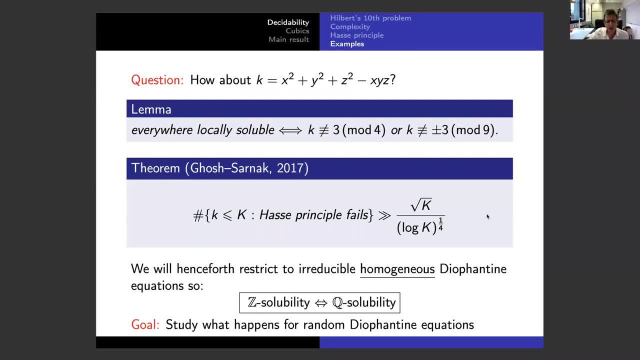 by Goshen Sarnak a few years ago, who actually proved for this particular equation that there are infinitely many counter examples to the Hauser principle. so it'd be interesting to figure out what's going on in these kinds of cases, and I think this is not. 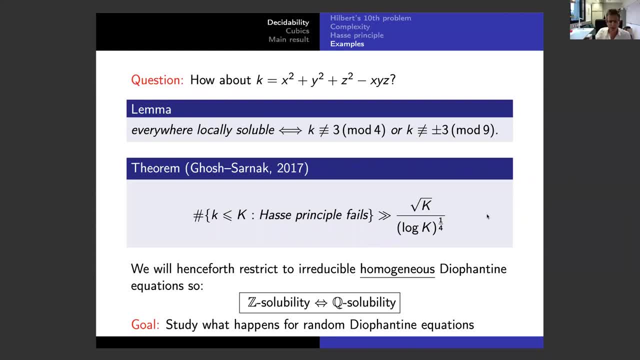 completely understood. so for the rest of the talk I'm going to talk about irreducible, homogeneous Diophantine equations. so all of them, all of the monomials, have the same degree, and this has the effect that talking about solubility over the integers is the same thing as talking about solubility of the 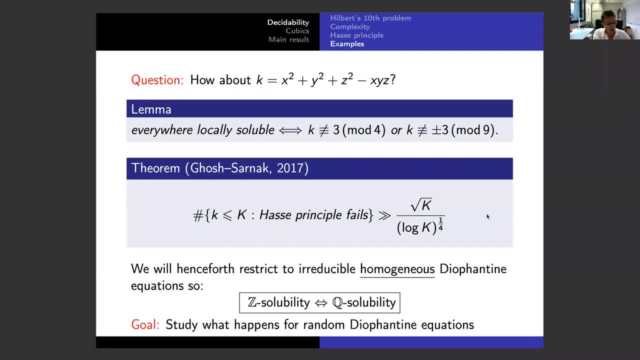 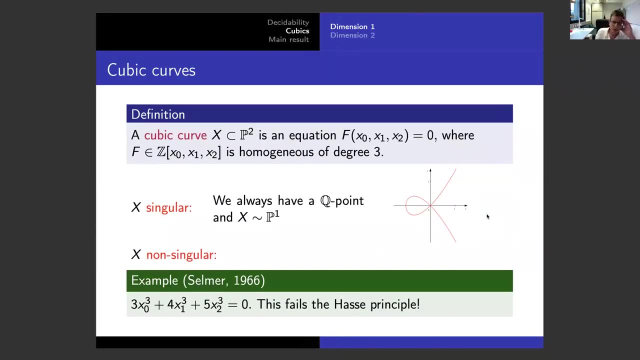 rational numbers and the motivation is going to be to ask about this test that I wrote but I don't contribute to, so we'll come to that in another lecture if we do end, because we also had a very long introduction as we were at 3 and I work. 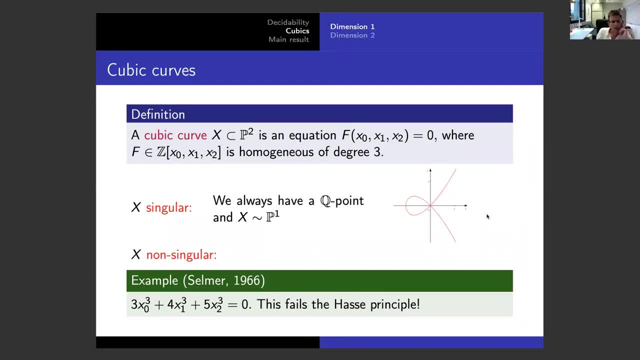 on the current project, where we're going to talk about components such as Hauser's algebra and the activities of Hauser's in one of our other engaging program on the topic of finite numbers So ended. I'd like to start by not talking about this limit that I've inibex сюда. 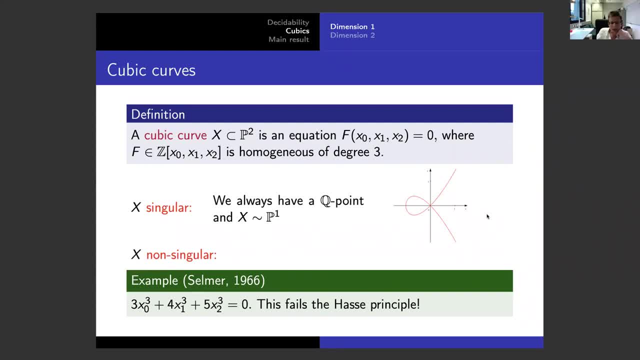 problema ro till schneller numeratorу for random equations. and the bit at the bottom to크를 homogeneous. so one of the mantras in diophantine geometry is that the complex geometry of the variety cut out by the equation, the polynomial equation, should have a very strong effect on the arithmetic of the problem. and we see: 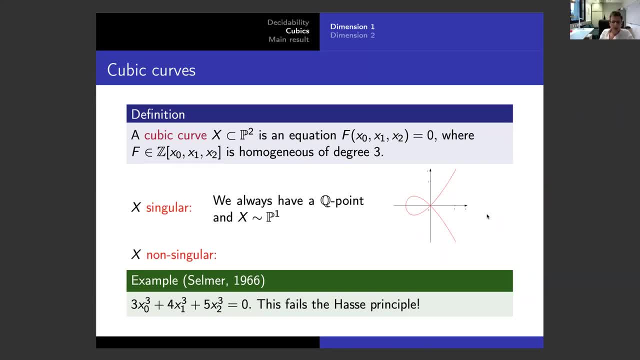 this quite distinctly here. so the problem is very easy if you've got a singular cubic curve, so first of all, if you're, if your curve is irreducible, you, it's not hard to see that you always have a unique singularity. if there were two singularities, two double points, then the line joining the two double points. 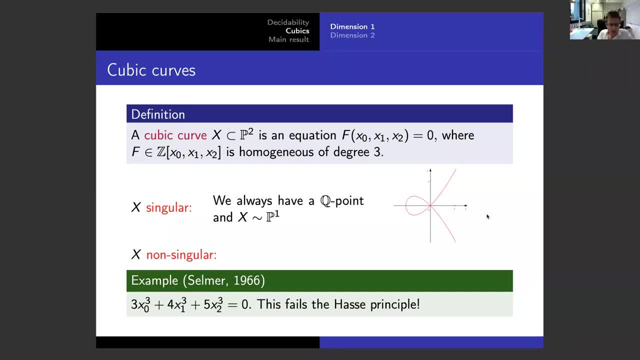 would hit the cubic curve in four points, which is impossible by pursuit's theorem. assuming the curve is irreducible, so it contains a unique singularity, you- and then by this singularity has to be invariant under the Galois group, and so this is actually always going to be a rational point on the cubic curve. so 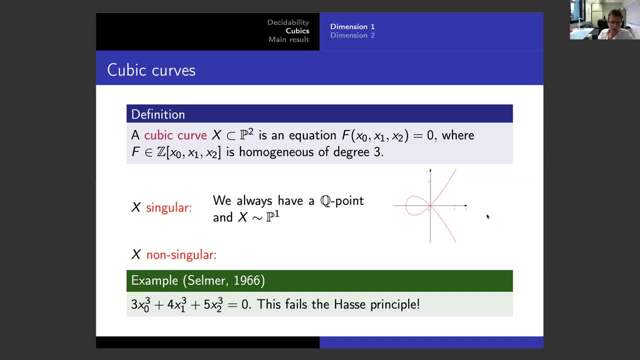 singular cubic curves always have a rational point and the fact you can use this rational point to parameterize all of the rational points and find that your curve is really just a copy of p1. things are much, much more subtle for non singular cubic curves and there's a 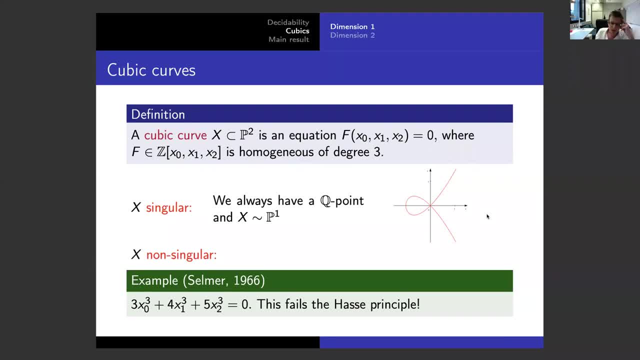 famous thing about this is: it is very hard to say what the actual product is, of example here of cell match- I'm sure you've seen before- which shows that this local test is not sufficient in general. so it doesn't. there are failures of the house of principle. 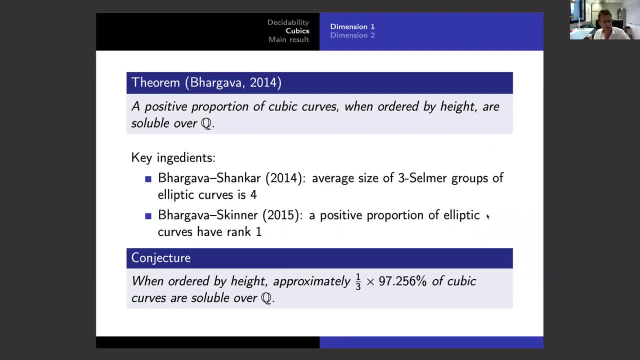 Let's move to dimension. oh no, stick with curves. Individual curves, difficult to analyze. so many questions about them. Vargava started seriously looking at answering these types of questions on average, and this will motivate what comes later. So this is a result I like a lot, and he has proved that if you order all ternary. 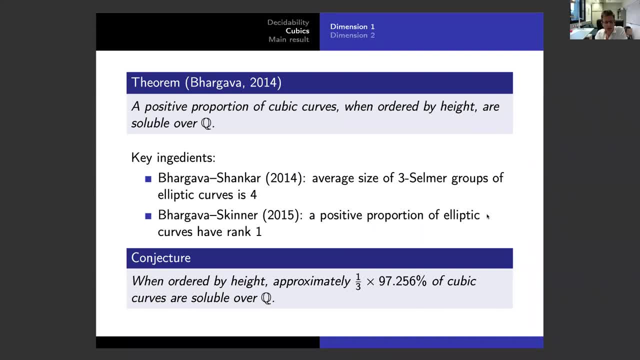 cubic forms by height, so ternary cubic forms over the rational numbers. by height, then a positive proportion of these actually have non-trivial solutions over the rational numbers. So this is a tour de force which builds on his work with Shankar on the average size of three Selmer groups of elliptic curves and his work with Skinner. 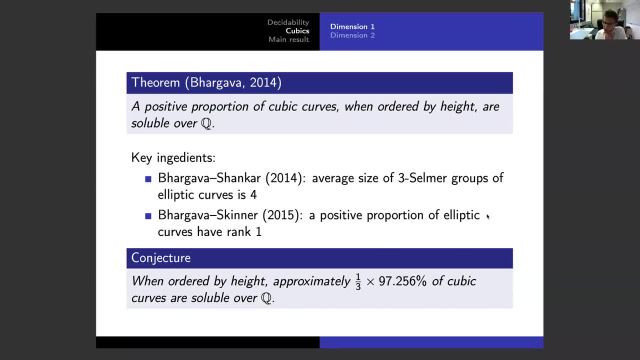 showing that a positive proportion of elliptic curves actually have rank one. So in the paper he also postulates a conjecture that I've written it in a fairly strange way. but the exact proportion of cubic curves which have a rational point should be one-third times. 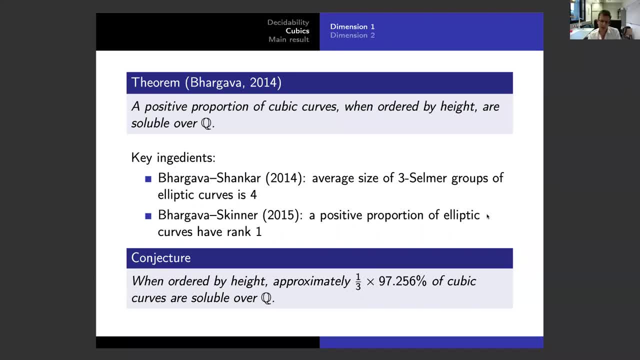 0.97.. This should be the proportion of cubic curves which have a rational point, not just the number of curves. So the point 0.97 actually comes through joint work with Mangiel and John Cremona and Tom Fisher, where they calculate the exact probability. 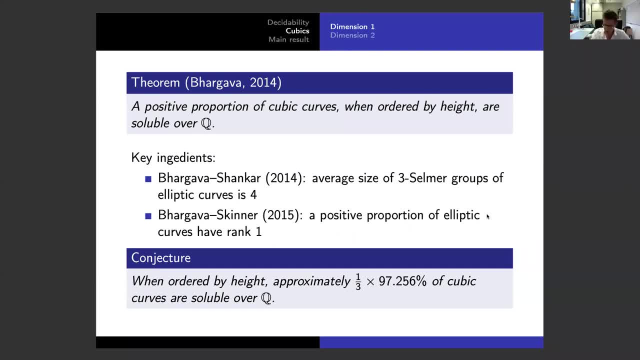 that a ternary cubic form passes all of the local tests, so it's locally soluble everywhere. So 97 percent of plain cubic curves are everywhere locally soluble, and among these Vargava conjectures that precisely a third of those actually have rational points. 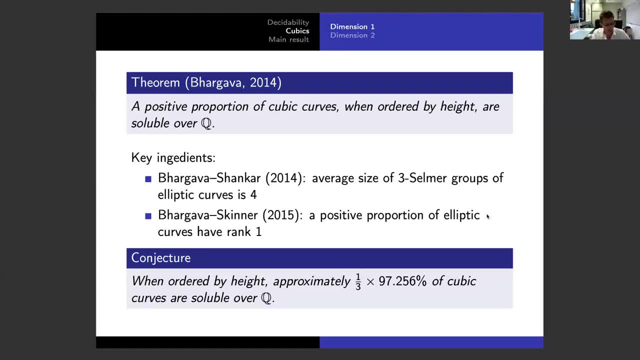 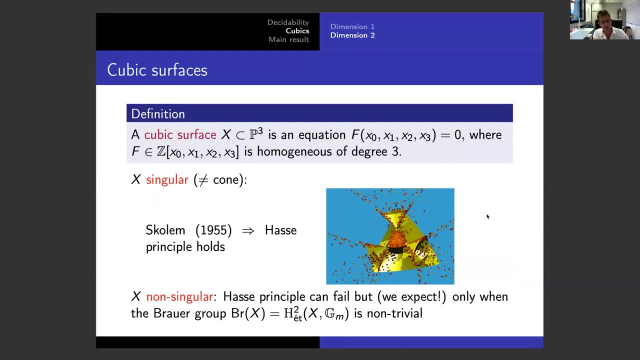 so this third sort of comes out of the method and is related to sort of rank distribution conjectures of Goldfeld, Katz and Sarnak. okay, so now I think we're moving to dimension two. so cubic curves were homogeneous. cubic polynomials in three variables, cubic surfaces: 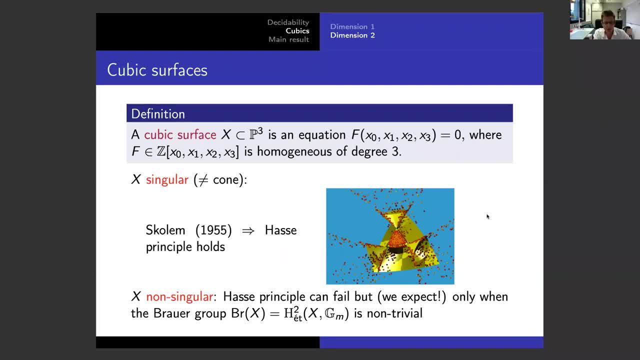 are homogeneous cubic polynomials in four variables and again we have this dichotomy between singular and non-singular surfaces. so the singular ones are easier, provided you stay away from cones. I think cones over genus one curves will be no easier than looking at the arithmetic of genus one curves. 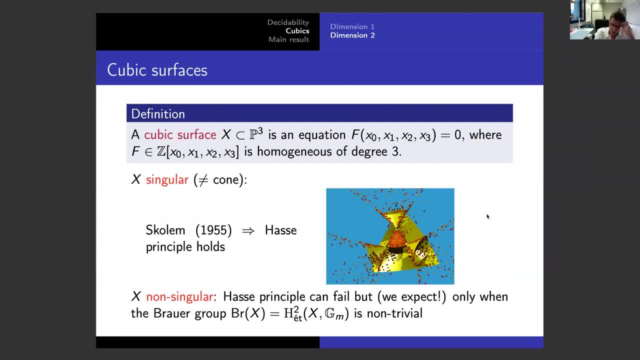 but so the geometry of singular cubic surfaces is very classical. you always have at most- assuming it's a normal cubic surface- you always have at most four singularities. it was proved over 50 years ago that the Hassa principle always holds for these cubic surfaces. I've illustrated one of my favourites. 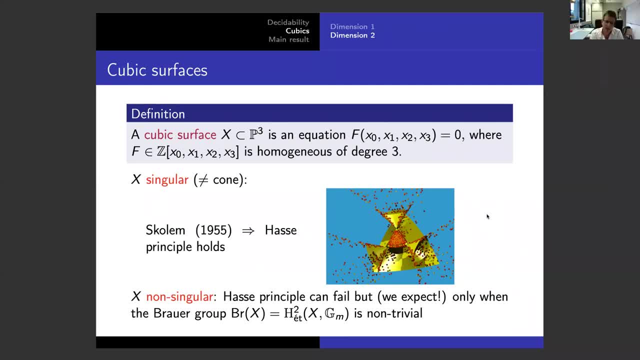 this is the Cayley cubic surface. it has this: this is the- the maximum number of singularities, and it has a bunch of rational points on this cubic surface. So the non-singular cubic surfaces are much more recalcitrant. We know that the Hasse principle can fail. 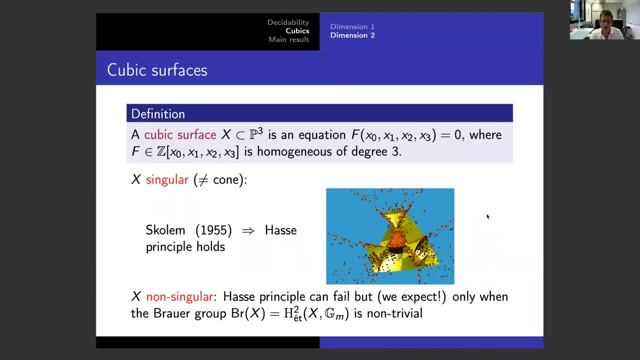 for these cubic surfaces. but we expect- and in fact this is a conjecture of Sansouk and Collier-Tillen from the 1980s- that the only way that it can fail is if the Brouwer group associated to the cubic surface is non-trivial. 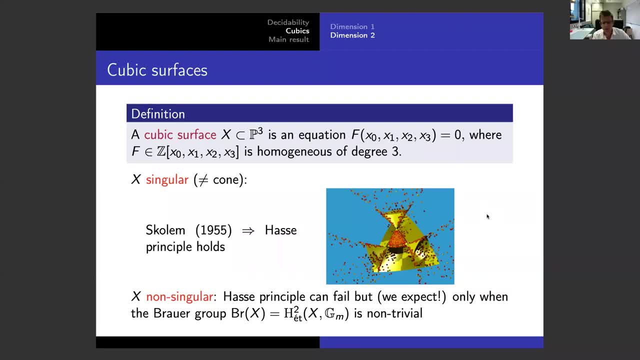 Whereas for singular cubic surfaces, we've had some success at even understanding the distribution of rational points on those cubic surfaces, Non-singular cubic surfaces are much harder. I've 3D printed. I don't know if you can see my video. 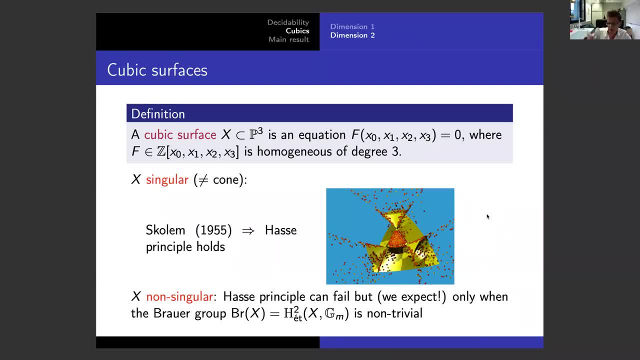 but I've 3D printed a cubic surface Here. this is the Klebsch cubic surface and all the pink dots correspond to rational points on this cubic surface. We have very little idea about how they're distributed. I mean, we have lots of conjectures. 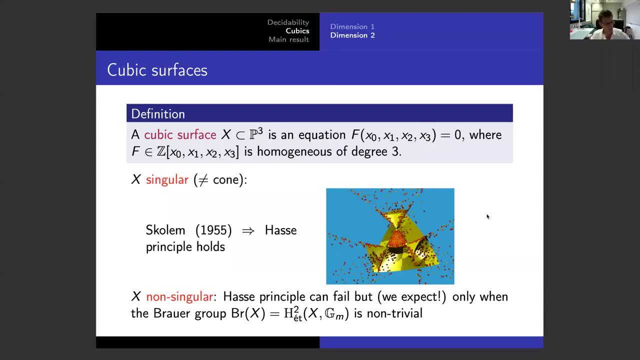 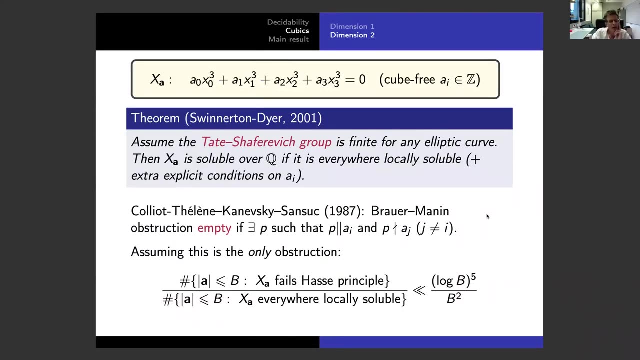 but relatively few proofs. So I wanted to point out that, yes, well, sort of underline the point that understanding individual, non-singular cubic surfaces is difficult. So this is one of the strongest results in this direction that we have. I'm focusing attention on diagonal cubic surfaces. 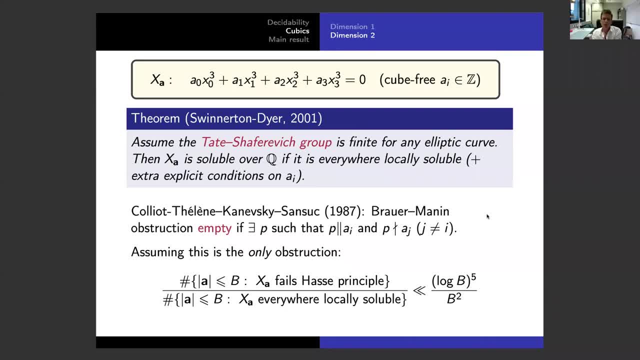 so I assume that it just has these four cubic monomials and they're all cube-free, And Swindon and Dyer, at the turn of the millennium, was able to show that these cubic surfaces admit rational points, assuming that they pass all of the local tests. 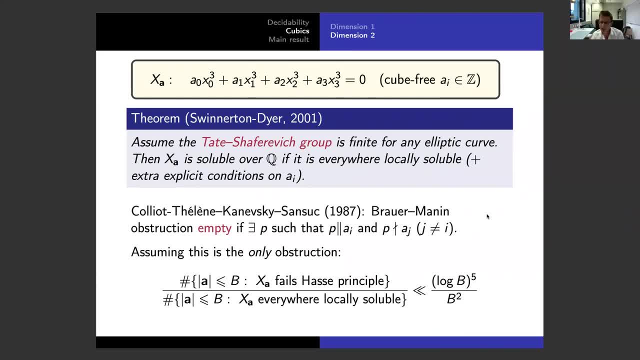 for solubility, plus some extra explicit conditions on the coefficients, which I'm not going to record, but you will find that here. So that's a there's a very strong result, but, as with many of these results in this area, 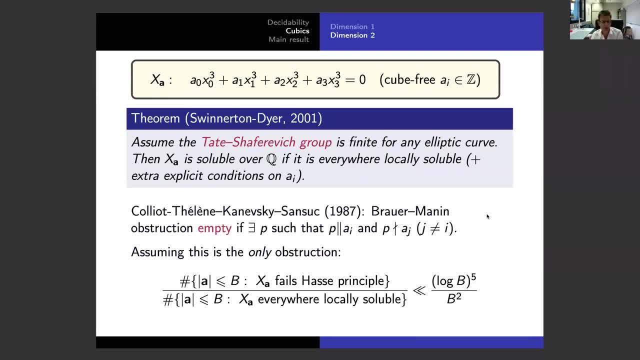 it's highly conditional. So he has to assume that the Tate-Savarevich group is finite for any elliptic curve. That's a big open problem in number theory. So in the 80s Kaliotulen, Konevsky and Sonsuk made a detailed study of diagonal cubic surfaces. 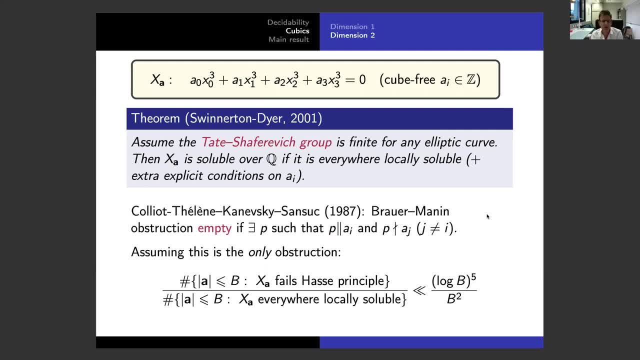 Explored what the Brouwer group or the Brouwer-Manning obstruction has to say about solubility for these surfaces, And so the calculation- one of the calculations they did was to show that This obstruction is empty, So there is no obstruction to. 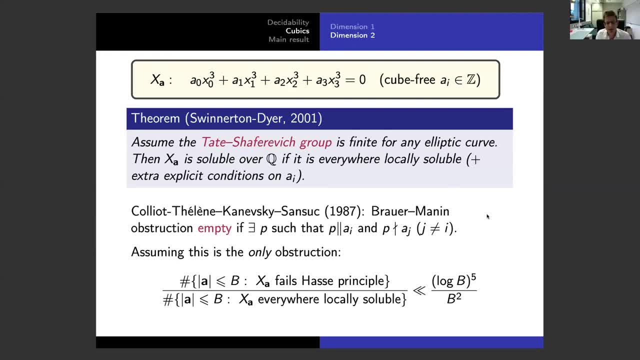 the Hasse principle, if Well, whenever you have a single prime P which divides One of the coefficients to the first power to Pianic valuation, one, and doesn't divide any of the other coefficients. So one consequence of that is that failures of the Hasse principle in this particular family should be exceedingly rare and 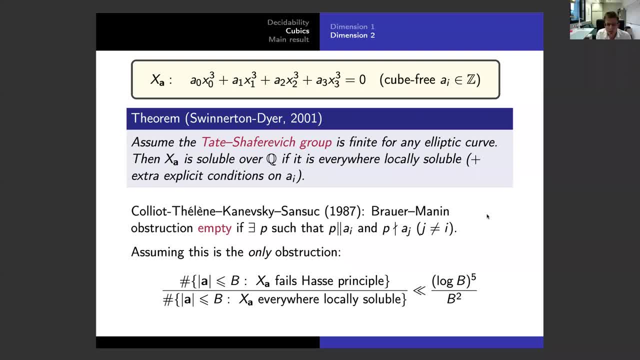 if you think about it, you can only possibly have a Brouwer-Manning obstruction if, Whenever there's a prime dividing one of the coefficients, either it's Square divides the coefficient or it divides another one of the other coefficients and That places a very strong multiplicative constraint on the coefficients. That's not very hard to show that. 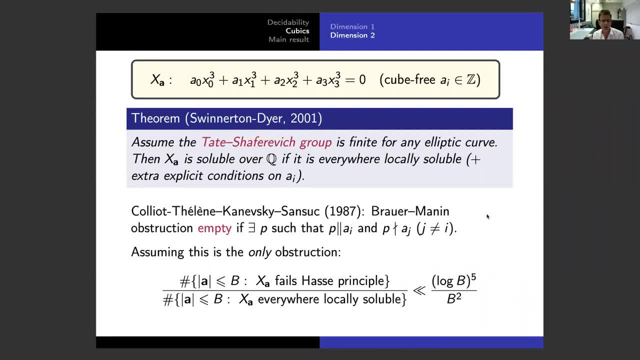 Well, assuming this big conjecture that the Brouwer group explains failures of the Hasse principle, that the proportion of failures should be Decay like 1 over B squared, and That's not going to be a very good result Nonetheless. So this is a sort of conditional result about cubic surfaces, but it is still possible to prove. 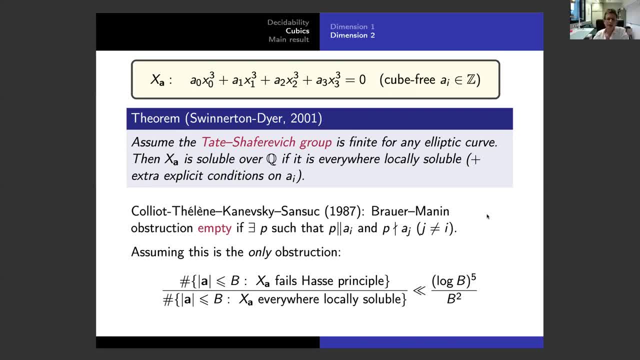 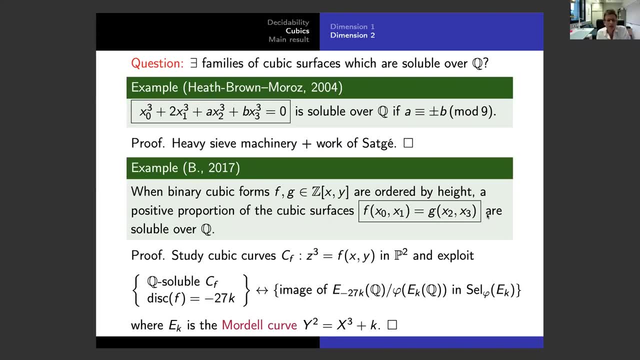 unconditional results about Existence of rational points on cubic surfaces and In fact you're able to prove Examples of families of diagonal cubic surfaces for which we always have a rational point. so there's a result by Heath brown and morales Which states that if you have the coefficients 1 to a, B, 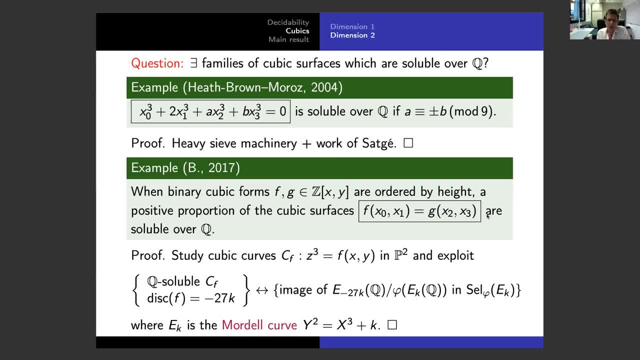 and we assume that a is congruent to plus or minus B mod 9, Then this cubic surface always has rational points. So this, this is really a, a sort of high point of marrying, sort of heavy analytic machinery with sort of work on Hegener points in. 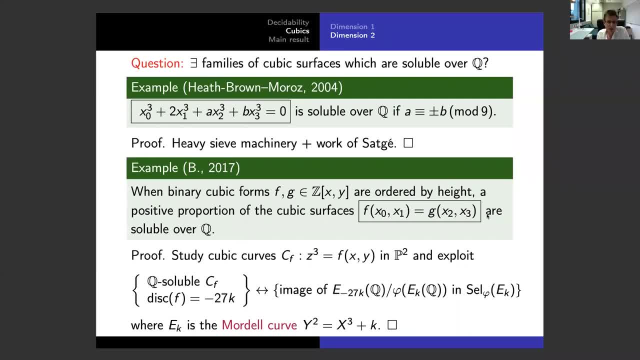 elliptic curves. So there's a result by Satche who shows that the cubic equation x naught cubed plus 2x1 cubed, equal to p, for a prime p congruent to 2 mod 9, always has a rational point. So if you're able to produce prime values of your 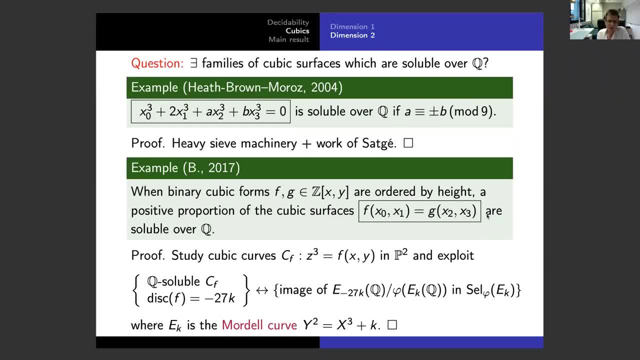 binary cubic form in the right congruence class, then you're able to deduce the existence of rational points on this surface. So I was sort of inspired by this and by the works of Bhargava to think about a similar family. So here I'm. 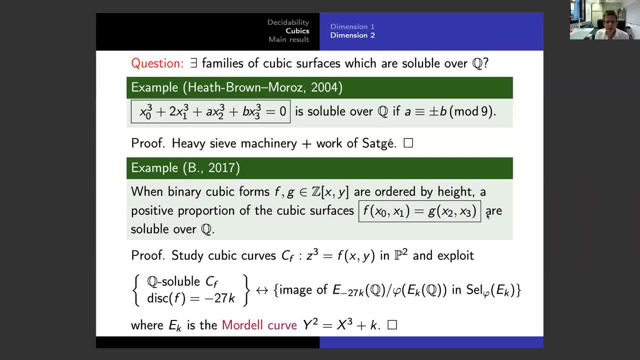 looking at a family of cubic surfaces which are of the shape binary cubic form, equal to a binary cubic form in disjoint variables, And one can show that in this family a positive proportion of them actually have rational points, basically by reducing it to a problem about curves in. 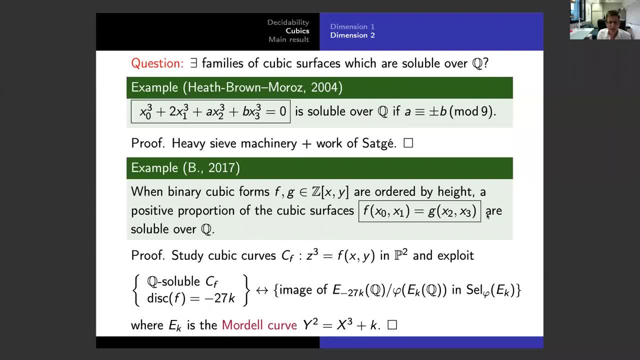 a fairly obvious way. So, in the same spirit of the Heath-Brown-Morales paper, it's sufficient here to just study the, the cubic curves in p2 which look like binary cubic form equal to a cube, And then you can exploit a connective. 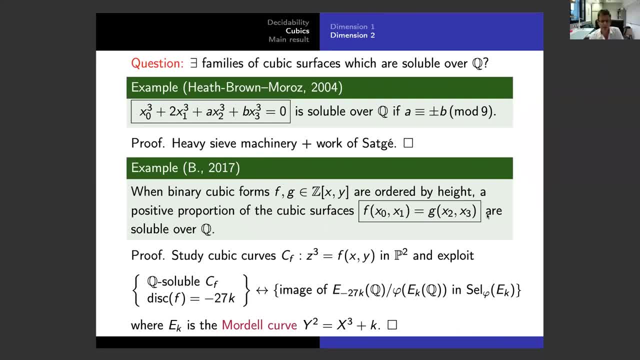 connection with these J invariant zero Mordell curves And one finds that soluble cubic curves of this special shape with given discriminant actually correspond to the image of this E mod phi E in the phi-Selma group of this Mordell curve. So this curve has a sort of obvious 3-isogeny. 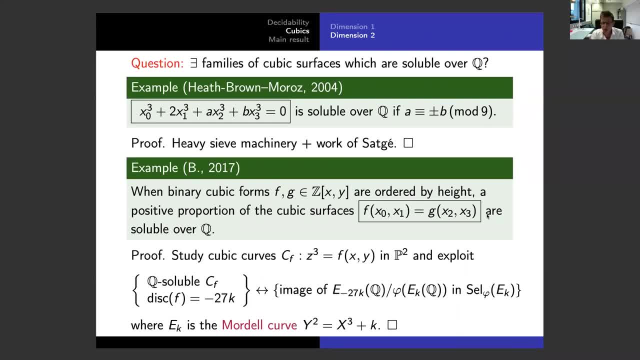 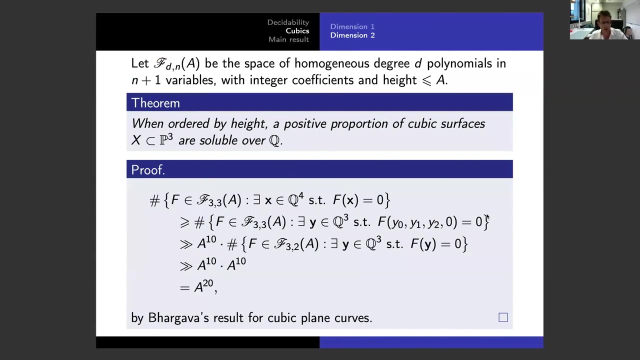 And then you can appeal to work of Chris and Lee, who actually are able to show unconditionally that a positive proportion of these Mordell curves have positive rank. Okay, so let me stick with cubics for a little bit longer and under the philosophy that any 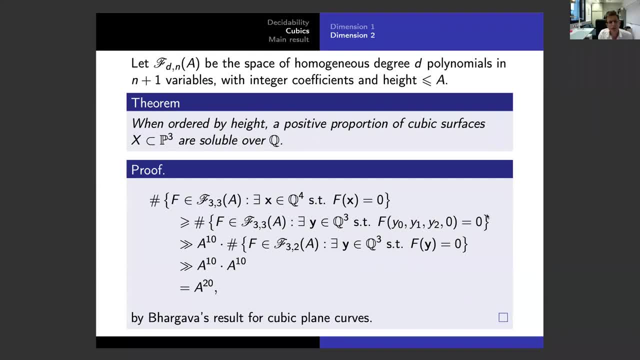 mathematics talk should always contain a proof. Let me present the following result. So I want to introduce some notation which will be used later as well. So curly f of a with subscripts d and n, This is the space of all homogeneous degree d polynomials in n plus 1 variables with integer. 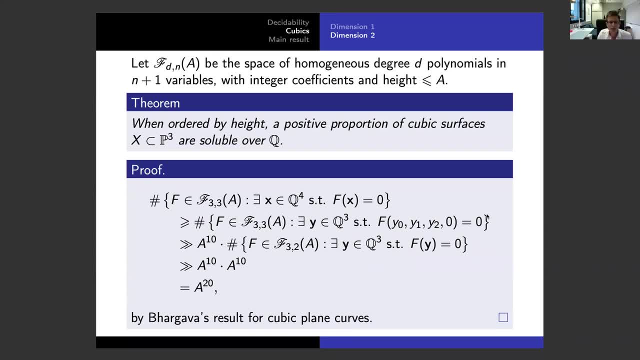 coefficients and whose coefficients all have modulus at most a. So a here is a parameter that will be tending to infinity. So the theorem it's about cubic surfaces is that when you order these cubic surfaces by height, you actually get that a positive proportion of them are soluble over the rational numbers. 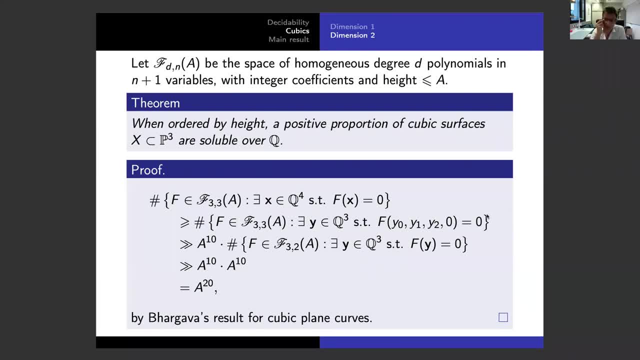 Okay, so that sounds like quite an impressive result, but it follows very easily from from Bargevay's result about cubic curves that I mentioned earlier. So we're interested in estimating the number of cubic polynomials, cubic forms, in four variables which have a rational. 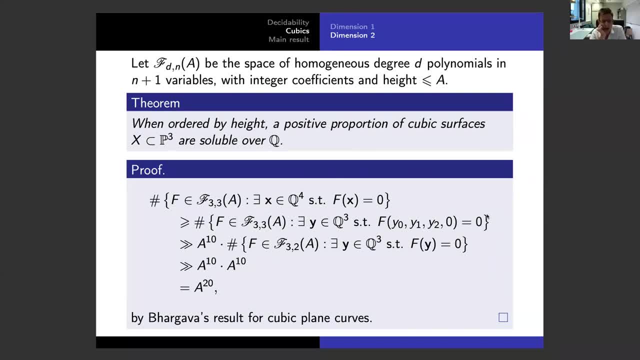 solution. I can lower bound that by just counting the number of cubic polynomials in four variables which have a rational solution in which the last variable is zero, the last coordinate is zero. So there are 10 monomials in cubic surfaces which have which involve: 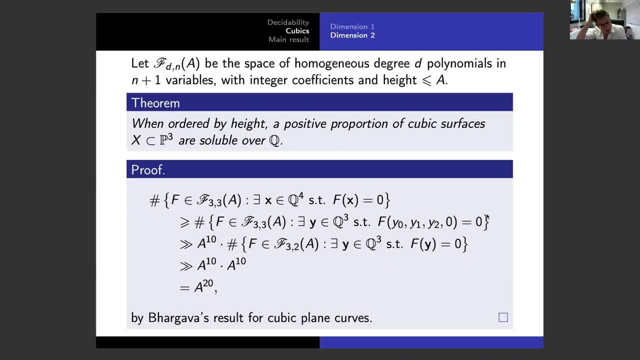 the x3 variable. So I can easily. so I essentially have a free sum over 10 of the coefficients and I get a lower bound of the shape greater than greater than a to the 10,, no greater than a to the 10,. 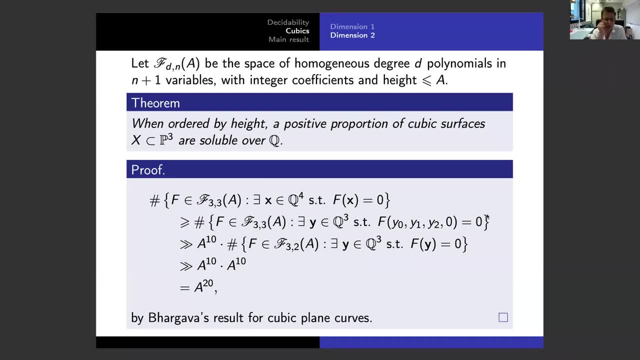 now times the number of cubic polynomials in only three variables which have a rational point or have a rational solution, and that's exactly the content of Bhargava's result, and he showed that there was a positive proportion, which just means that there's a lower bound of the. 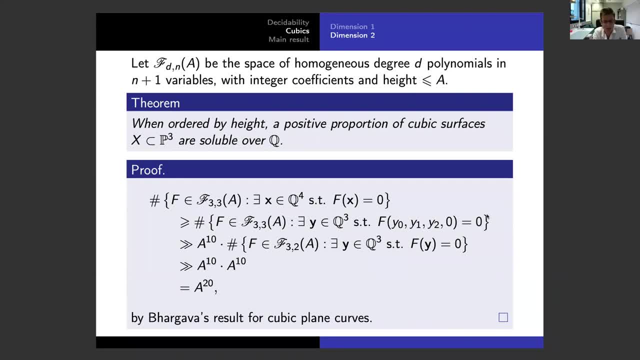 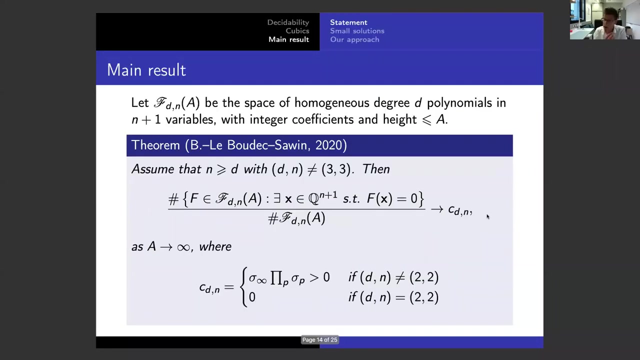 shape of constant times a to the 10.. There are 10 monomials in any cubic polynomial in three variables, And so that gives you the result. Now let me get on to talking about the main result that we've been working on. So again, it's the same same notation as before. Curly f is the space of all of these. 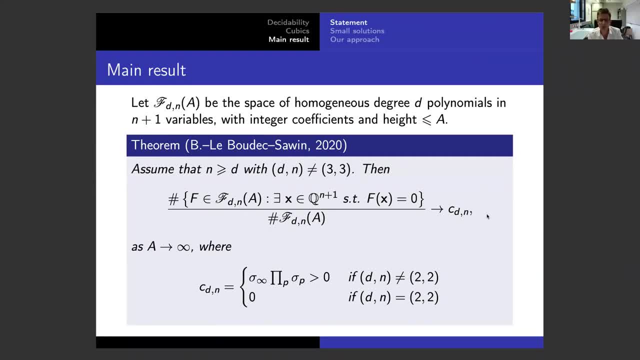 homogeneous degree d polynomials in n plus one variables with integer coefficients and height at most a. So then the result is that, provided that we're in the so-called Fano range, so the number n should be at least d, And we have to exclude the case of cubic surfaces, the case d and n being three. 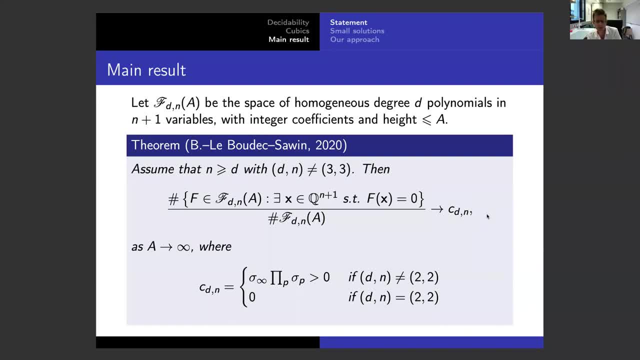 And that's OK. it's unfortunate, but we have to exclude the case of cubic surfaces. Then the proportion of polynomials which have a rational point tends to a constant: c, sub d, n, as a goes to infinity, And this constant has a nice description. 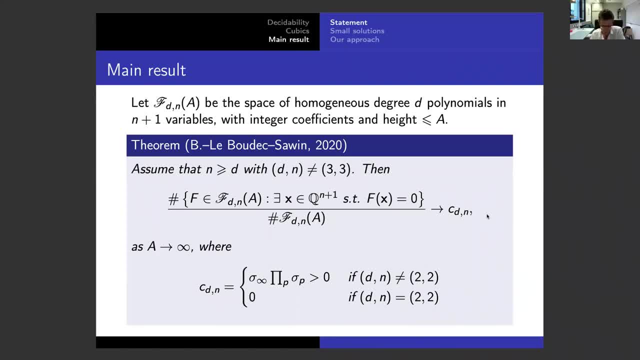 If you're outside the setting of plane conics it admits a description as a product of local densities and a positive product of local densities, And if you're in the setting of plane conics, this constant is zero. So that was already well known. That's a nice result of say from the 90s that a random plane conic doesn't have any rational points. 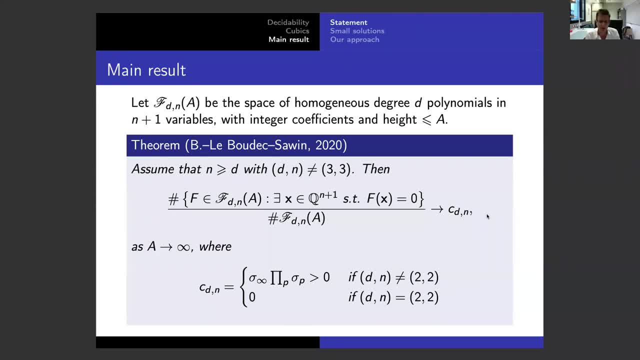 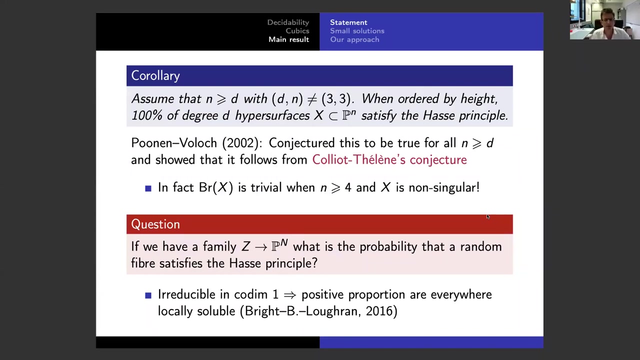 So I won't define these densities here. but sigma p, for example, is the probability that a homogeneous degree d polynomial in n plus one variables has a q p point. So another way of saying this is that, again, if you make the same assumption, so n is at least d. 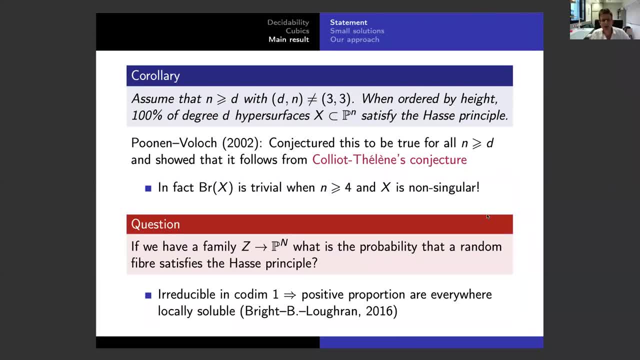 We're not looking at cubic surfaces anymore. When you order these all by height, 100% of them satisfy the Hasse principle. Okay, so, while previously we saw some instances of counterexamples to the Hasse principle, this is at least confirming that these counterexamples are rare for this range of n and d. 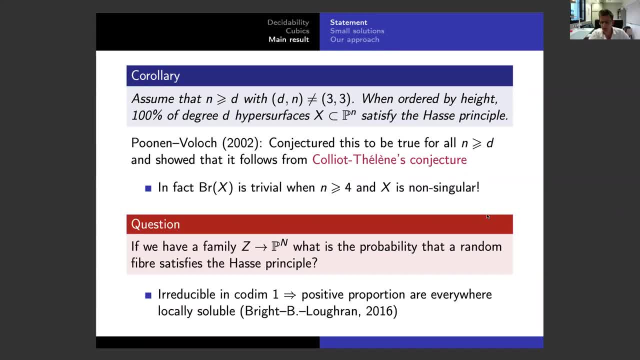 So, in fact, this question or this result goes back to a question or to a paper of Poonen and Volokh, and this influenced me a lot. I think this was just when I was finishing my PhD. It was a conference, one of my first conferences. 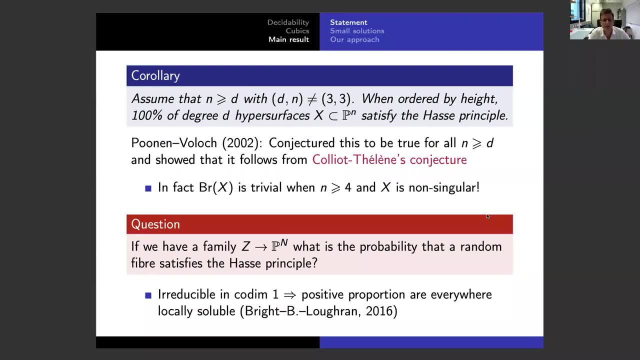 at AIM about rational points, And this was one of the things that was discussed there. So they made this conjecture that it should be true for all n greater than or equal to d, including cubic surfaces, And they also had a nice argument which showed that. 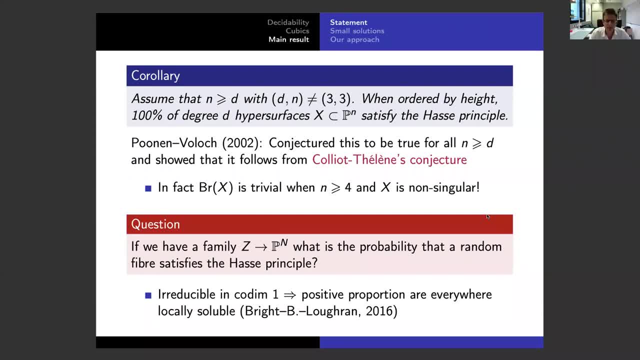 it follows from a very general conjecture of Collier to Lenn. So if you've not seen that conjecture before, that states that if you have any rationally connected variety, the Brown-Mannan obstruction should be the only obstruction to the Hasse principle. 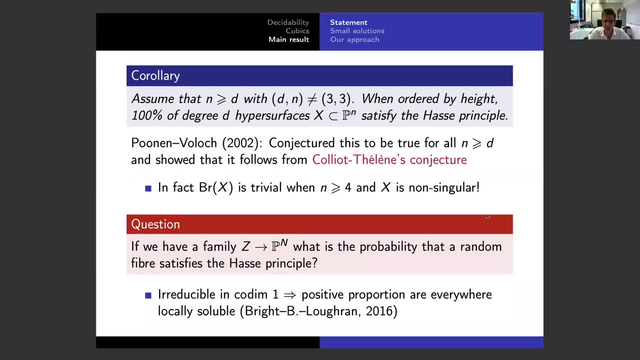 So if you take that on faith, actually it tells you something much stronger. in the setting of Fano hypersurfaces, because one can show that if n is at least 4 and x happens to be 0, which happens to be non-singular, 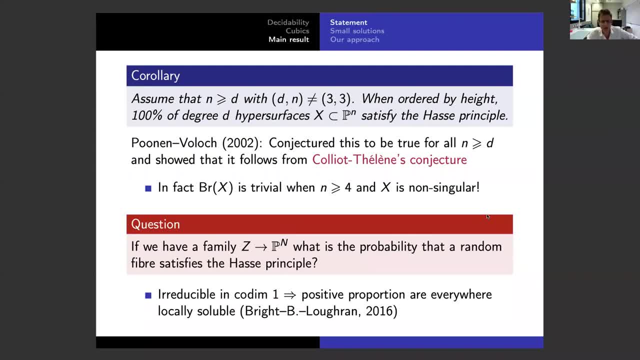 which certainly happens 100% of the time, then this Brauer group is trivial. So therefore, according to the conjecture of Collier to Lenn, the Hasse principle should always hold. Actually, in the light of that, it's possibly interesting to comment on the error term in this theorem. 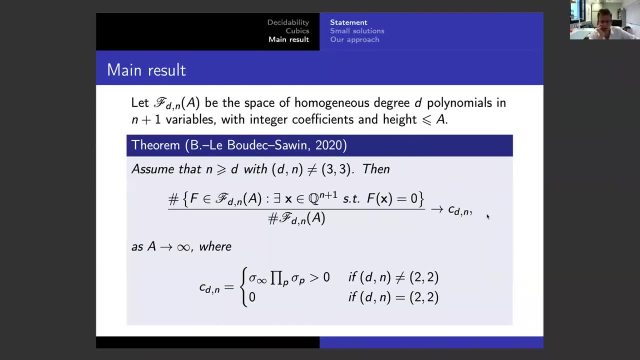 I suppose, if it follows from this argument based on Collier to Lenn's conjecture that this should be true for all n greater than or equal to d, certainly with an error term which is polynomial decay in A. So we're not able to obtain polynomial decay in A in this result. 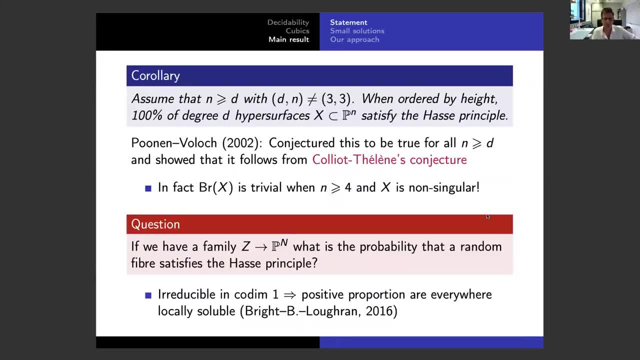 but we do at least get some explicit power of a logarithm, I guess. as I was preparing these slides, it occurred to be interesting to think about what one might expect in a slightly more general context. So if you give yourself a family, you have some smooth, projective variety z. 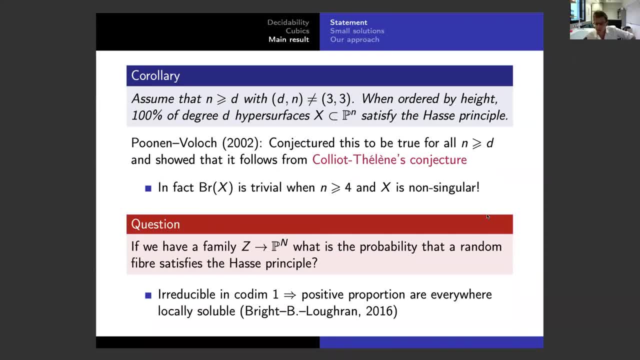 with a morphism down to some projective space. one might ask about what's the probability that a random fiber satisfies the Hasse principle. So I think it really only makes sense if you put some conditions on the family. So I'm assuming that. 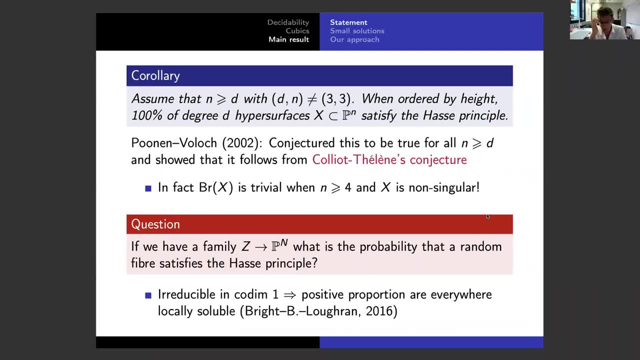 z itself is everywhere. locally soluble seems to be a fairly basic assumption. I guess you would want the fibers to be rationally connected perhaps, But it'd be interesting to think about what one might expect here. So at least the local solubility condition. 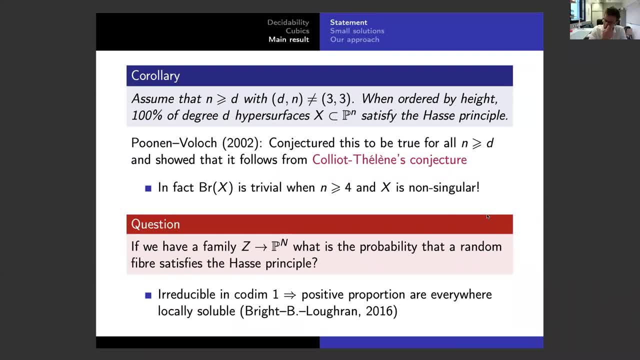 or result here has been worked out in joint work with Martin Bright and Dan Loughran. So if you assume that over every co-dimension, one point in such a family, the fiber is irreducible, then you can at least show that sort of using. 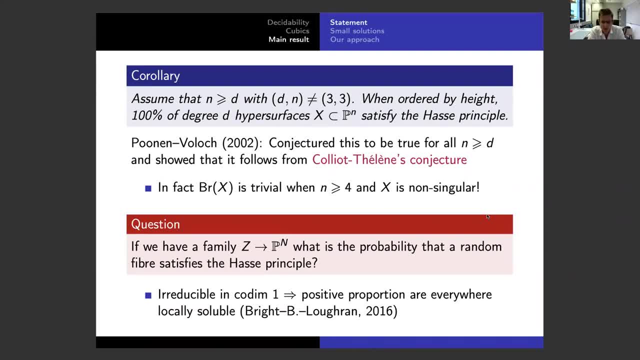 the sort of Sivavecadal type machinery that a positive proportion of the fibers are everywhere locally soluble. I don't know, Is this condition enough to guarantee that it satisfies the Hasse principle? I haven't thought about that, Okay. 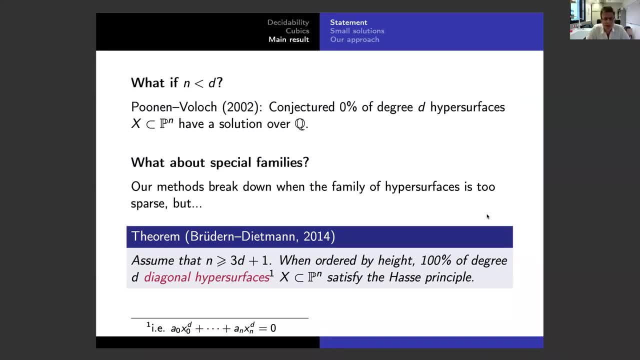 Maybe I should discuss a little bit about n less than d. Okay, so that's completely off the cards. Poonen and Volokh also conjectured that if you're in the world of general type varieties, 0% of them should have a solution over q. 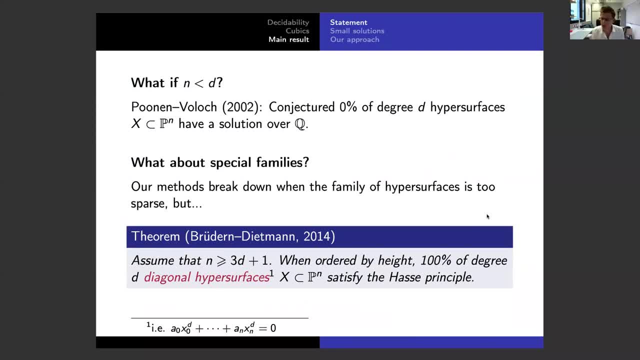 So interestingly here. it's certainly true that a positive proportion of them are everywhere locally soluble. So we expect failures of the Hasse principle to dominate. But even writing down a single example where the Hasse principle fails is very, very difficult. 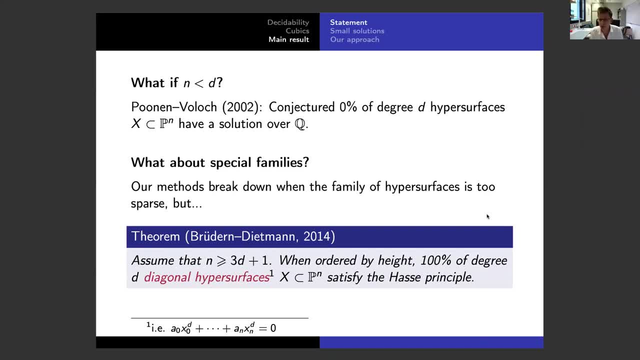 We have some results in this direction, but they're all conditional on things like ABC conjecture or other Bombieri-Lange type things. One could also ask about special families. So if the family becomes too special, then our methods unfortunately break down. 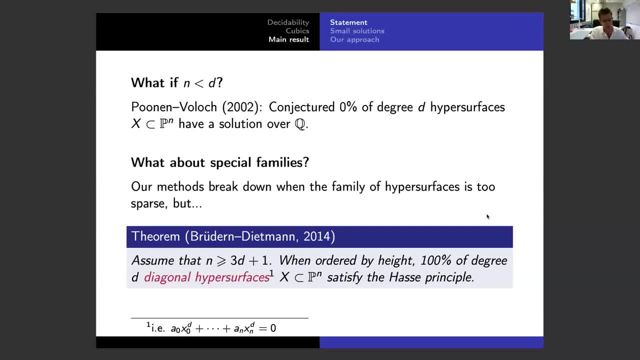 But there is some prior work in this direction. So Jörg Bruden and Rainer Dittmann considered the case of diagonal hypersurfaces And under a slightly stronger condition, on the relationship between n and d, so n is 3d plus 1,. 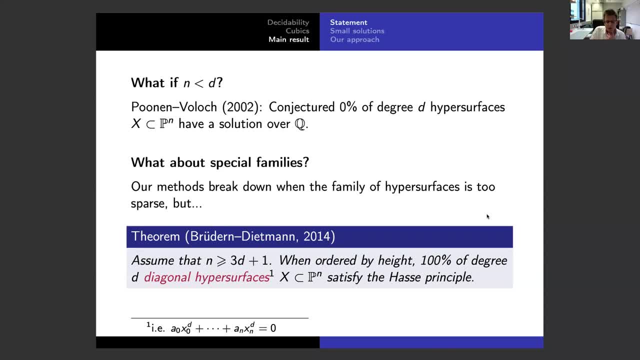 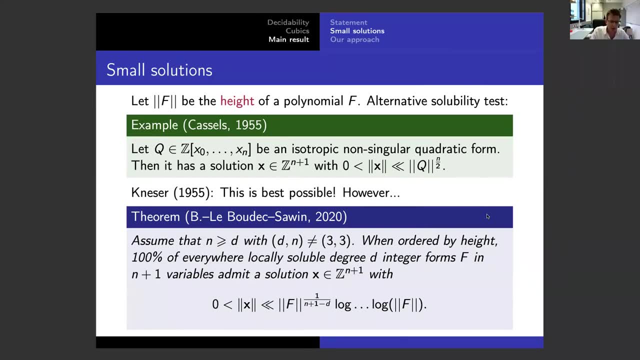 they're able to show that 100% of them satisfy the Hasse principle. Okay, so actually we're able to prove something slightly stronger than what I've revealed so far. We can say something about the existence of small solutions, So let me write double lines f. 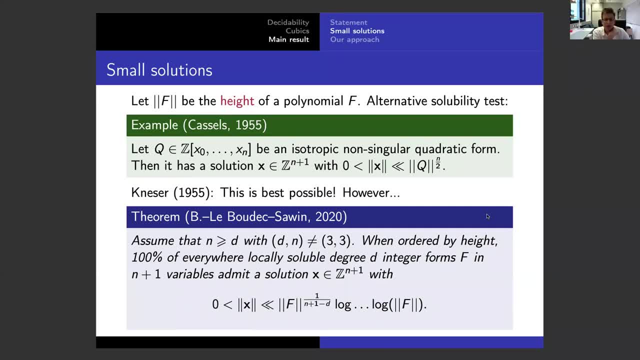 to be the height of the polynomial f, So the maximum modulus of the coefficients of the polynomial f. So there's a classical result of Cassell's about quadratic forms that states that if you have any non-singular isotropic quadratic form, then its least integer solution. 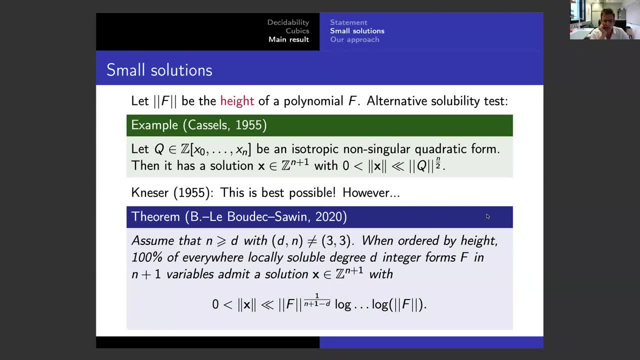 its least non-trivial integer solution always has Euclidean norm, at most at constant times the height of q to the n plus 2.. Sorry, n over 2.. So that's quite intriguing. So this gives a completely different sort of solubility test to the Hasse principle. 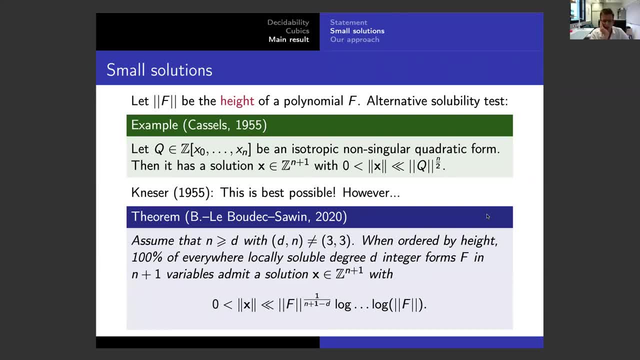 This is telling you that. I mean, if you wanted to know whether such a thing was soluble, you just have to run through all possible integer vectors up to this search range and figure out whether you have a solution or not. And there's been work on improving. 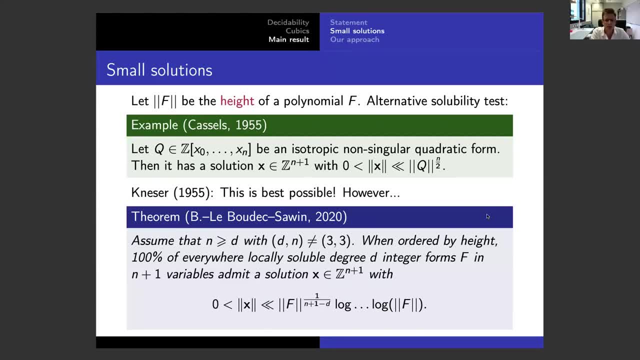 the implied constant, And by several authors, And in fact this is known to be best possible. So Knasser or Nasser, I don't even know how to pronounce his name- wrote down an example of a quadratic form which had large height. 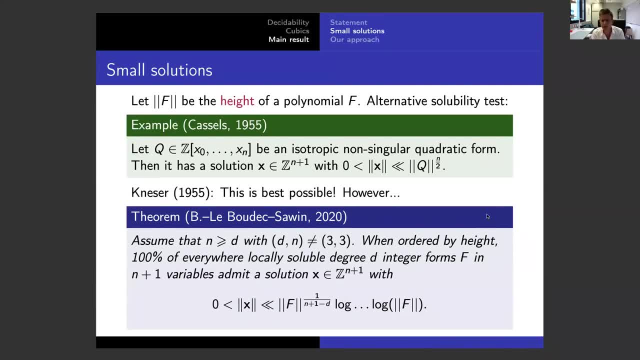 and whose smallest solution had large height, matching this upper bound of Cassell's. However, if you look at the equation he writes- sorry, the polynomial he writes down- it's of a very special shape. In fact, it actually has discriminant one. 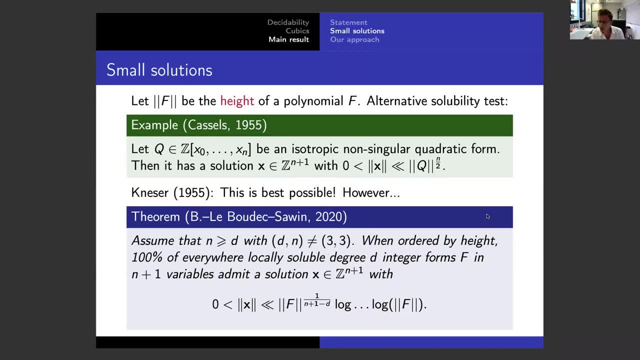 determinant one. So it's very atypical, So you might expect that on average, this isn't the true behavior, And this is sort of what we also managed to prove. So again, the same assumptions on N and D. N is at least D. 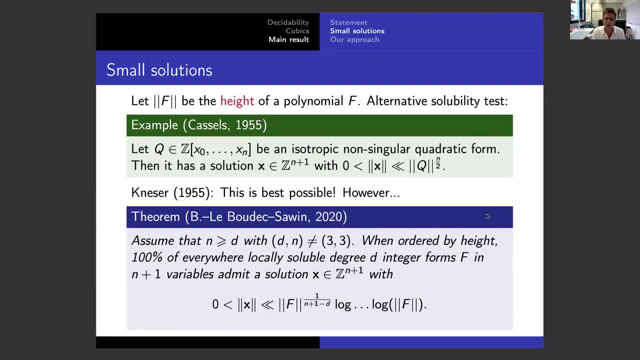 We're not looking at cubic surfaces, unfortunately, And so when you order everywhere locally soluble degree D integer forms in N plus one variables, then 100% of these have a solution in which the norm of this vector, the Euclidean length of this vector, 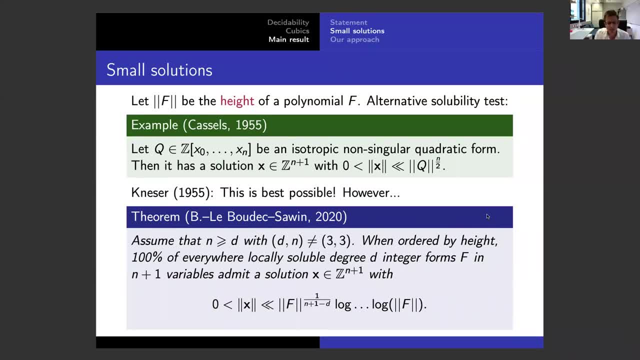 is bounded by the height to the one over N plus one minus D, times something that goes to infinity slowly. Yeah, so I promised there'd be some iterated logs. I think that's the only point at which they appear. So you can see that in the case, D equals to two. 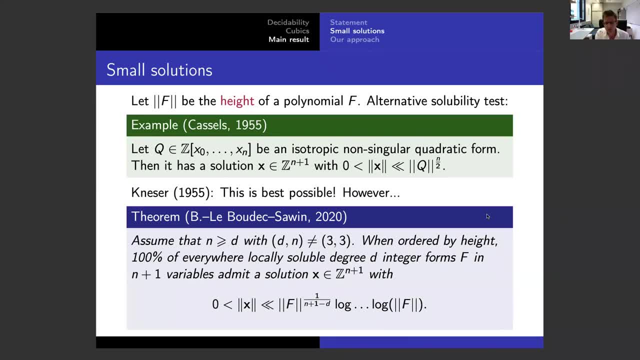 this is a much, much smaller upper bound than what we're seeing in Castle's result. Okay, So actually this chimes with work of Yuri Tchenko, Elzenhans and Yarnall, So they also postulated the idea that. 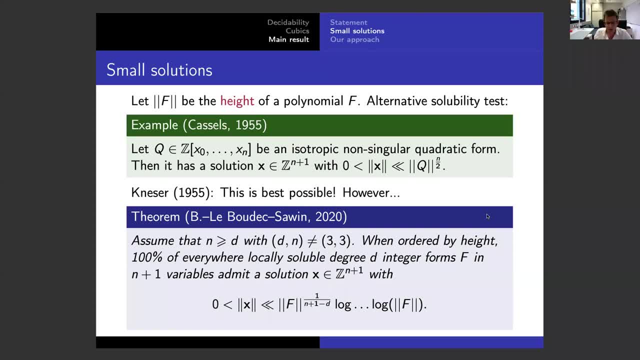 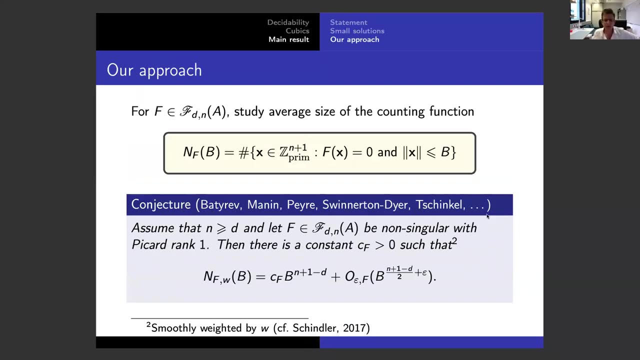 the point of least height on a Fano variety should be something like one over the Tamagawa measure, So it coincides with that, Okay. So let me talk a bit about our approach to this, So studying the question of which polynomials actually have solutions. 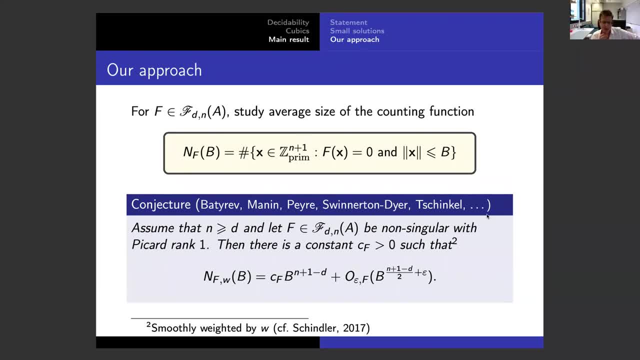 is quite hard to do And things are smoothed out a lot by instead studying the average behavior of the associated counting function. So we could define for a polynomial F, we could define N of B to just be the total number of primitive integer vectors in N plus one variables. 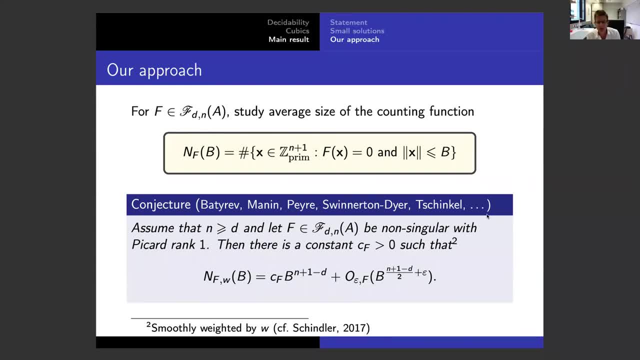 which are solutions to the Diophantine equation, F equal to zero, and which have norm at most B. So this is certainly a counting function that has proved my bread and butter for many years And I've thought about it in many different contexts And there have been 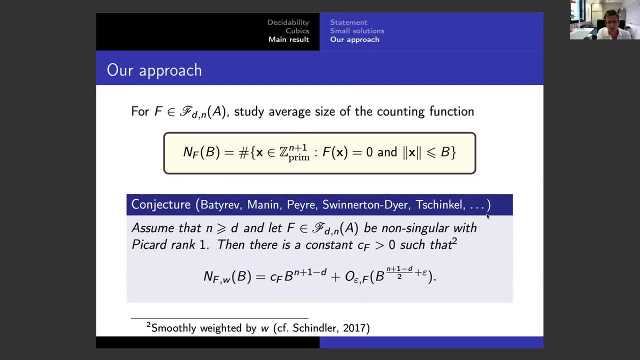 numerous incarnations of what one might expect for these kinds of counting functions. So here's a conjecture. It's sort of inspired by work of many people. If we take the Fano range, so N is at least D and F is one of these polynomials. 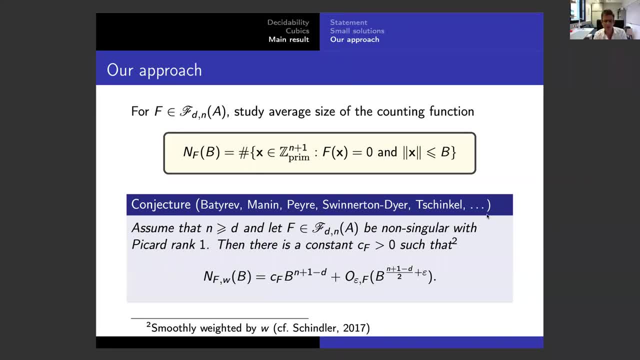 of degree D and N plus one variables. I'm going to assume that it's non-singular and that it has Pickard number one, So it's Pickard group is just Z. Then one might expect that there's a positive constant. All right, I need to assume. 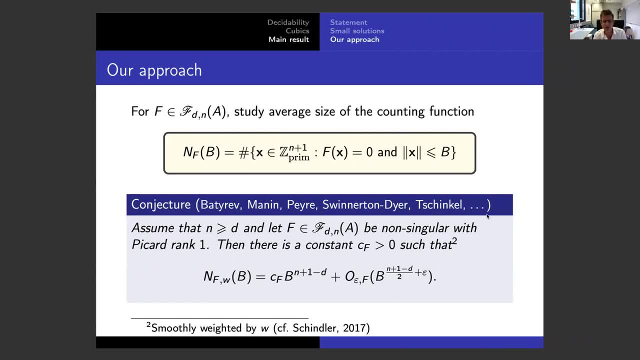 that it has solutions. Otherwise this problem is not very interesting. So I might expect that there's a positive constant such that this counting function behaves asymptotically like this: constant times B to the N plus one minus D, So there's a fairly easy. 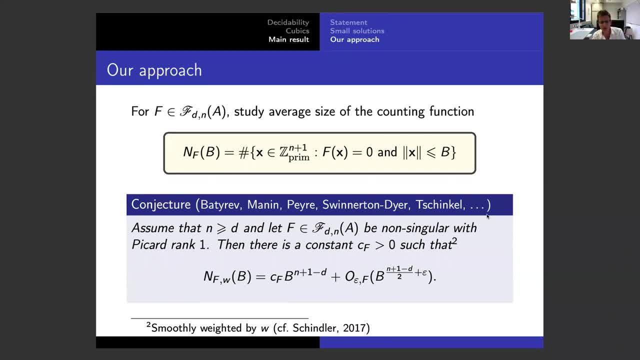 heuristic argument for explaining the exponent N plus one minus D. I think in your wildest dreams you might hope that, as in several other instances in analytic number theory, that you actually have a square root error term. So there's a paper of Swindon Dyer. 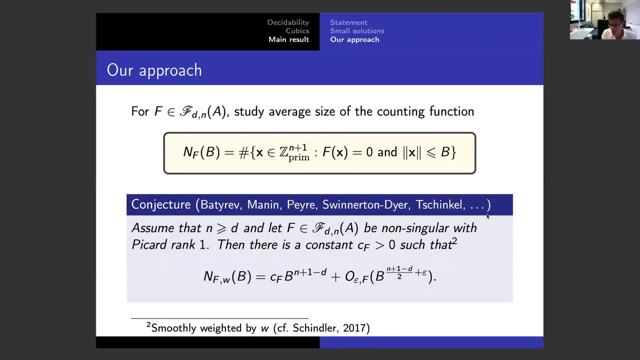 where he conjectures this for cubic surfaces, for example. I'm cheating here slightly because there are some issues around dealing with sharp cutoff functions. There's a paper by Damara Schindler who demonstrates that you can get sort of intermediate lower order terms. 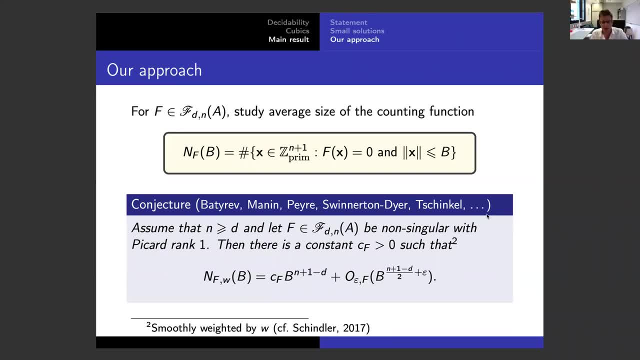 appearing in asymptotic formulae like this. But I think the consensus is that if you move away from some sharp cutoff functions to something smoothly weighted by some smooth weighted compact support, say, then those lower order terms go away. So maybe this is a reasonable. 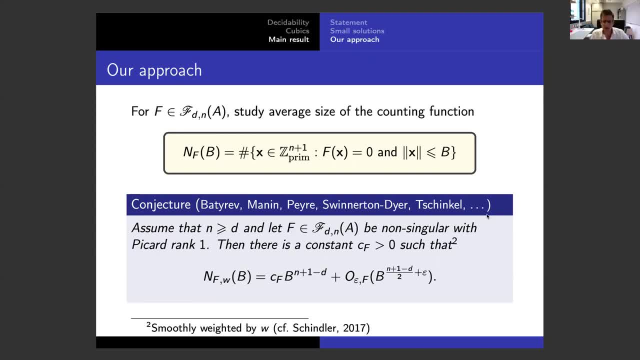 conjecture to hope for. In fact, it's probably worth. It'd be interesting, probably very, very difficult to think about. I mean, this is To think about this in the context of whether or not this error term, If you normalize the error term. 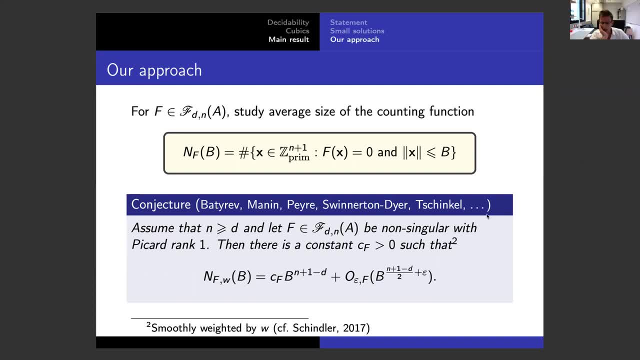 appearing in this asymptotic formulae. in the spirit of Zeb's talk a couple of weeks ago, where he talked about a conjecture of Blair and Dyson about sums of three squares, it'd be very interesting to see whether there's any evidence for this normalized counting function. 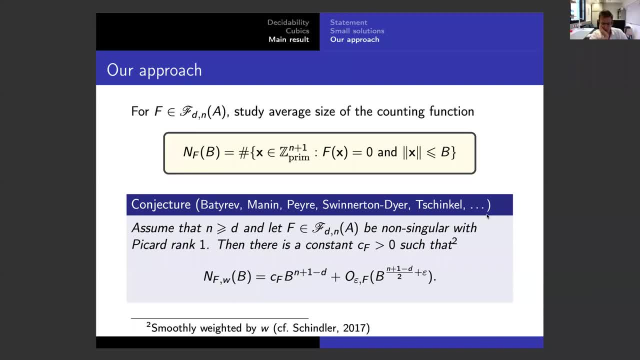 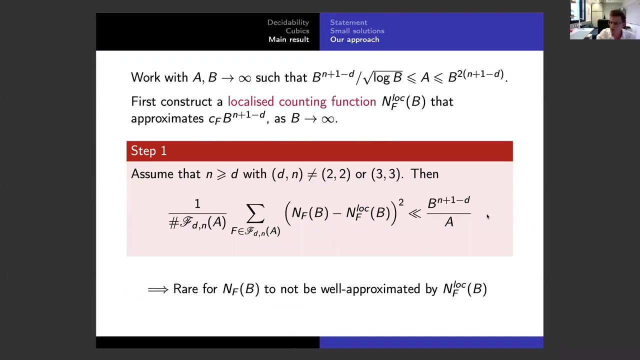 to have a limiting distribution, A normalized error term, to have a limiting distribution, Maybe a Gaussian distribution, Why not? But at least our work is consistent with this conjecture. So we basically have two parameters going to infinity, And what we're doing. 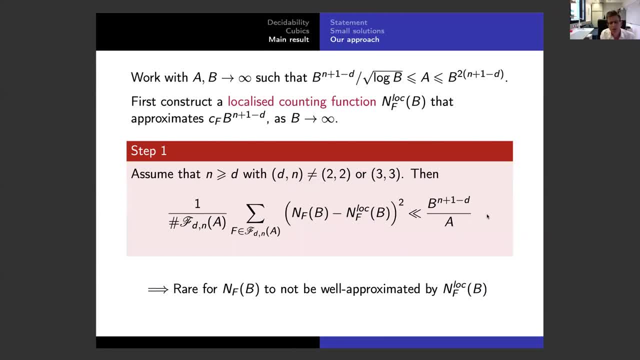 there's the a, which is the height of the polynomial, and then there's the b, which is the height of the rational solution to the equation. So we have to take a in a certain range with respect to b and all of the work is concerned. 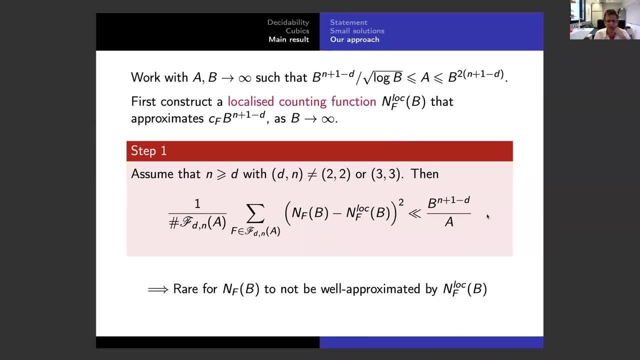 with dealing with the case where a is close to the left-hand inequality. So indeed, that's the situation where you expect there to be the fewest number of rational points. So the basic process or the basic point of view is to try and start by constructing. 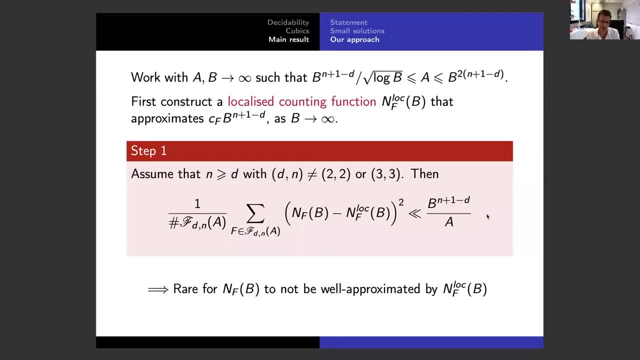 a convenient localized counting function which I'm just going to denote by n log of b. And this counting function has got to be rich enough. this localized counting function has got to be rich enough that it approximates our expectation for what the leading behavior should be. 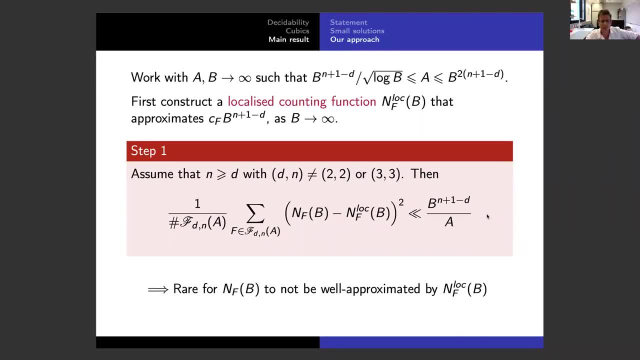 in the Manon conjecture, but easy enough that we can actually work with it. So that took a bit of doing to get that right. But you can essentially think of it as a truncated singular series and a truncated singular integral coming from the circle method. 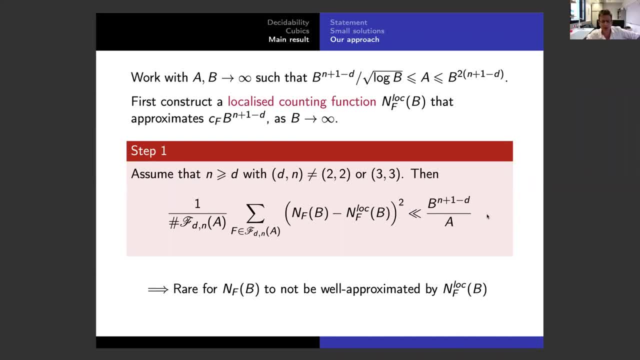 So the first step, and the most important step, is to study the mean square of the difference between the counting function and the localized counting function as we average over all of these homogenous polynomials of degree d in n plus one variables, And then the result. 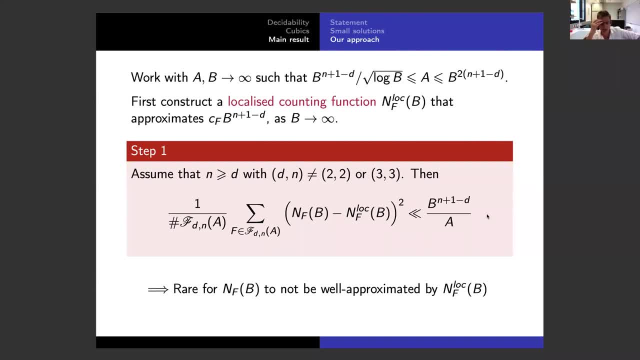 that we are able to prove is that, basically, we get a square root error term on average whenever we're dealing with this range. that n is at least d, And now we have to exclude the case of plain conics and plain cubics- sorry cubic surfaces. 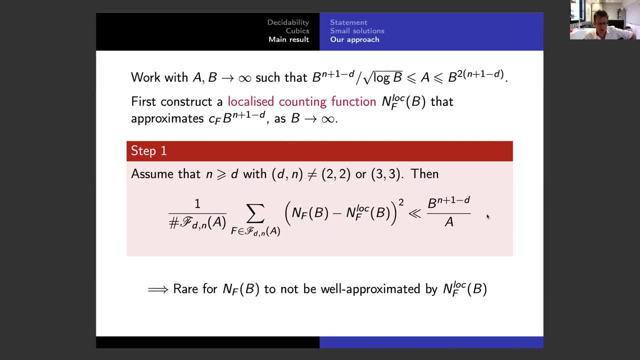 Yes, I think in earlier iterations of talks I've given about this we've been- I'll say a bit more about this in a minute- but we've been stuck at n being at least d plus one, n being at least d plus two. 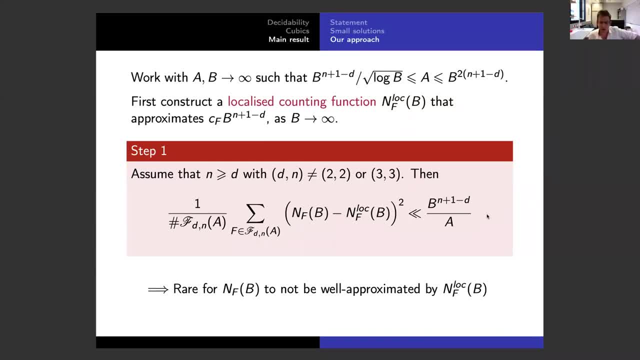 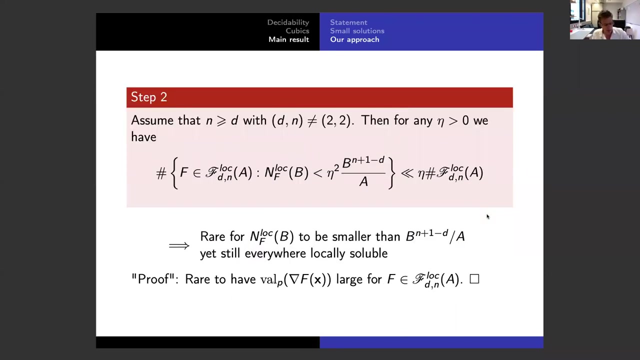 And handling the case n is equal to d becomes harder and harder as n and d gets smaller. Anyway, the upshot of this result is that it is rare for our counting function to not be well approximated by our localized counting function Now going hand in hand with that. 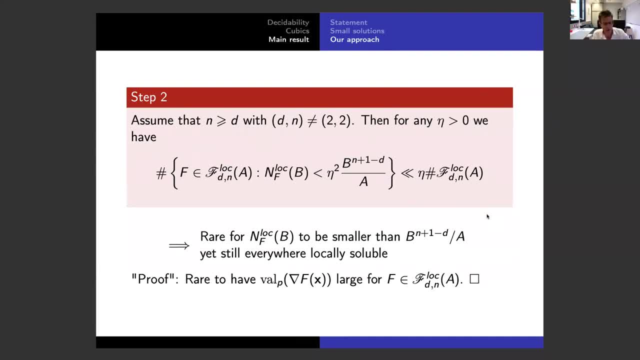 is an analysis of the localized counting function itself. So we want to show that it is rare for the localized counting function to be smaller than we expect it to be. Okay now, the one issue here is that actually we know that for a positive proportion. 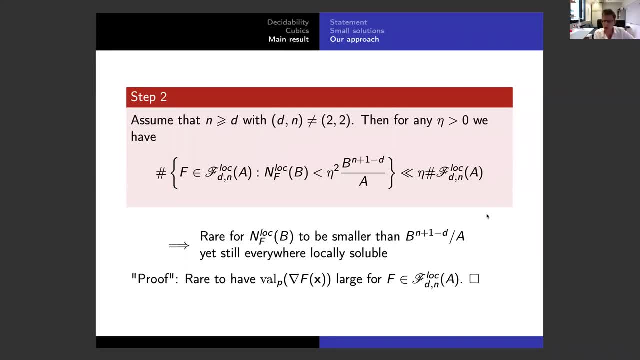 of polynomials of degree d and n plus one variables, this localized counting function vanishes. So it certainly can be small, And it's here that we really need to work, under the assumption that we're only restricting attention to polynomials which pass all of the local tests for solubility. 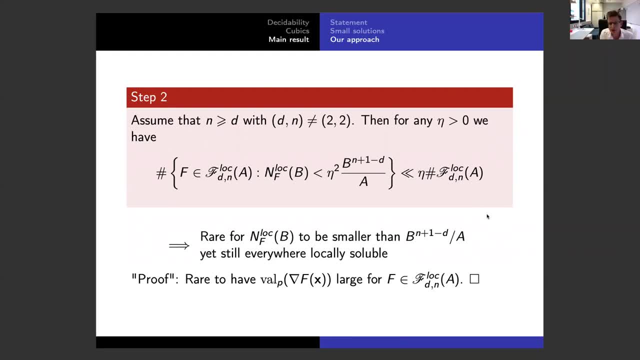 So we're looking at. so this curly F lock is now the restricted set of everywhere locally soluble polynomials of degree d and n, plus one variables and height a. So this estimate tells you that it's rare for this localized counting function to be smaller than we expect it to be. 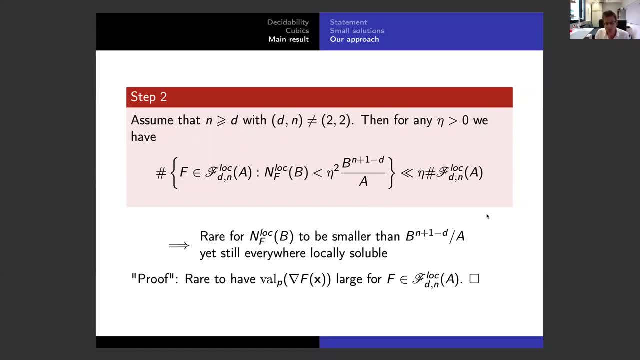 and yet still everywhere locally soluble. So I'm not going to talk about the proof of this, but it really goes back to what we saw on the second or third slide involving Hensel's lemma. So Hensel's lemma told us that 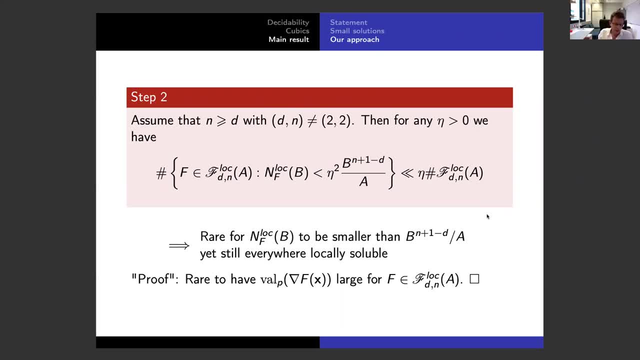 you know, when you're in a situation that the periodic valuations of the partial derivatives are small, then you can lift points. you can lift points to get many p-adic points on your hypersurface. So the guts of the argument here is to sort of show that. 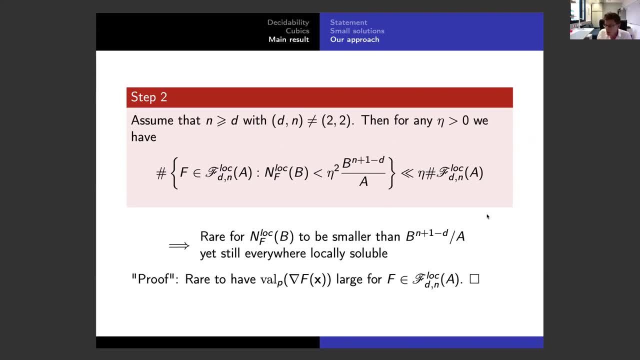 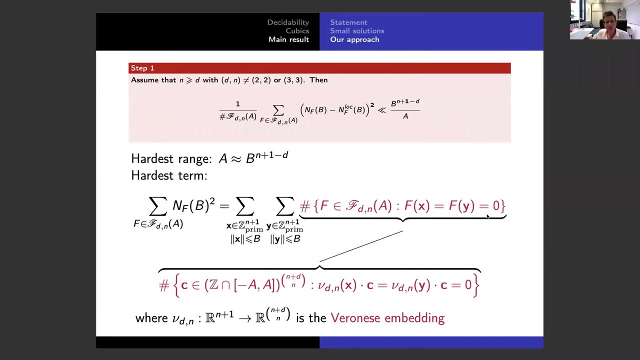 it's rare that you have polynomials which are locally soluble and yet have all of their partial derivatives featuring large prime powers. Okay, I wanted to focus a bit on the first step, because this is the bit that involves the geometry of numbers. I've just recalled what the first step is here. 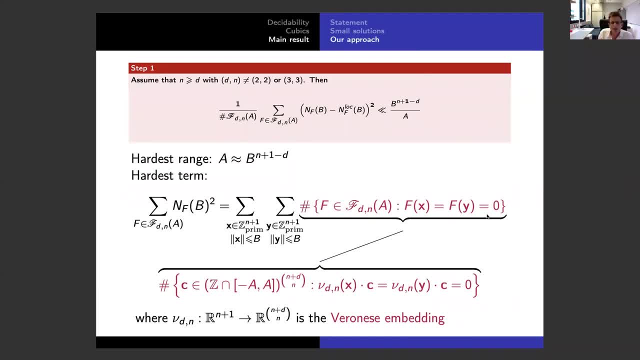 as a second moment bound, And the hardest range is, as you might expect, when a is roughly the same size as b, to the n plus one minus d. So that's the case in which the leading constant in the expected asymptotic formula for nf of b is roughly one. 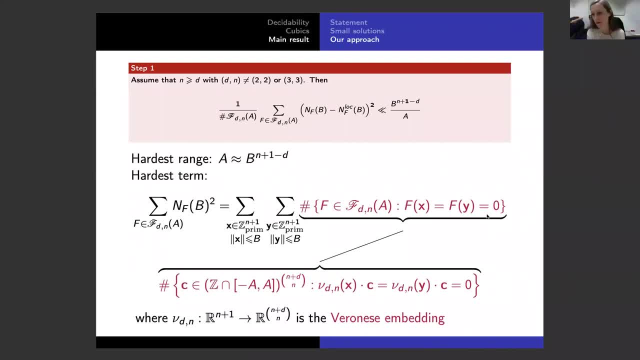 Tim, please excuse me. We have a question or a comment from Seth Rudnick. if you don't mind, Seth, please ask your question. Tim, so you have this two-parameter family and ideally you would like to make a very small relative to b right. 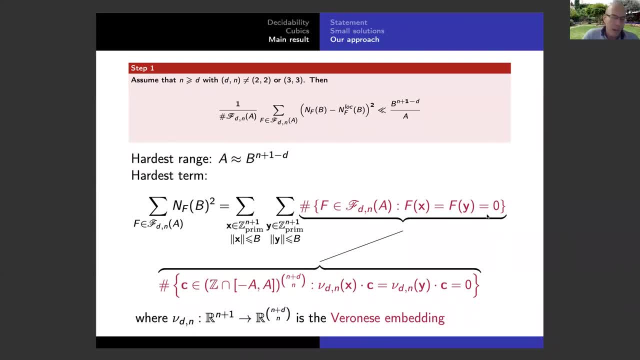 Because you're secretly trying to capture what happens for an individual hypersurface, right, But if I understand correctly, you are forced to take a quite large, which is, as you say, what you call the hardest range, That's, the lower bound. 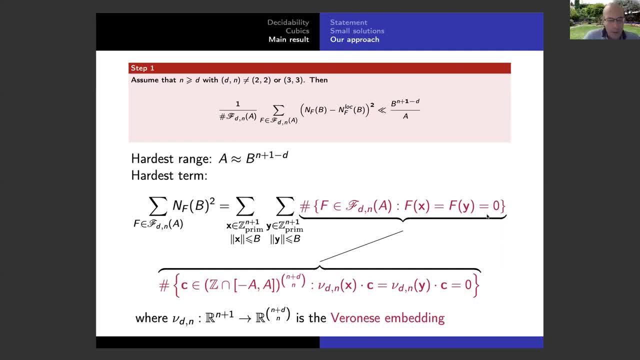 So you can't. And then you have this upper bound, which seems less important because, if I understand correctly, you want a to be small as possible. But if you give up on that, that upper bound, could you make a smaller than this power of d? 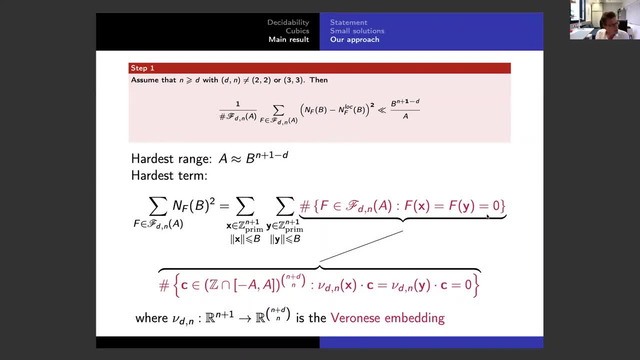 I get, I'm not sure. I think Yes, It depends what psychiatrists reject. Oh, certainly it will. Thank you, It depends what you're trying to prove, Like what? Wait, I made me confuse myself. You're talking about making a very, very, very small. 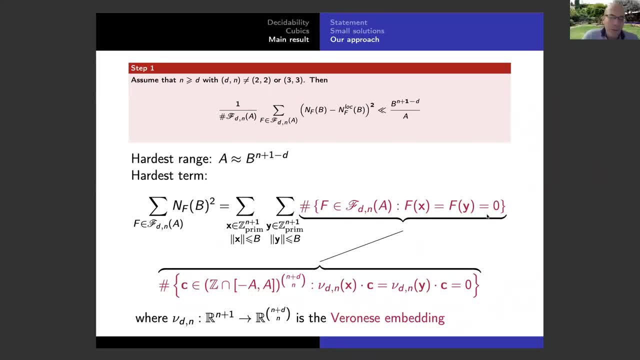 Or b, very small. Ideally you want- If I understand the philosophy you really are trying- Ideally you would want to do this for an individual, Yeah, A equal one- Yeah, Ideally. But of course we can't. 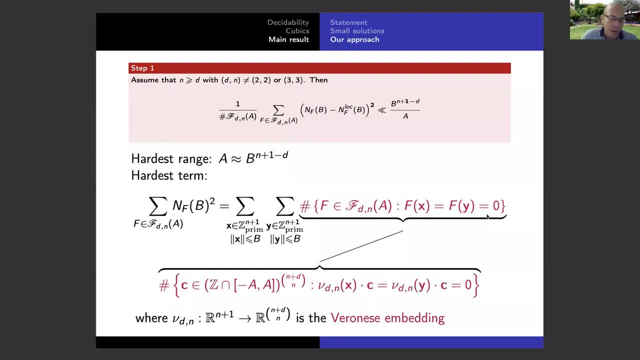 So you average, And so you try to average over as few possible hypersurfaces as you can, which means make a as small as you can, while still making it grow with b. That's a philosophy, I would imagine. Yeah, But your force? 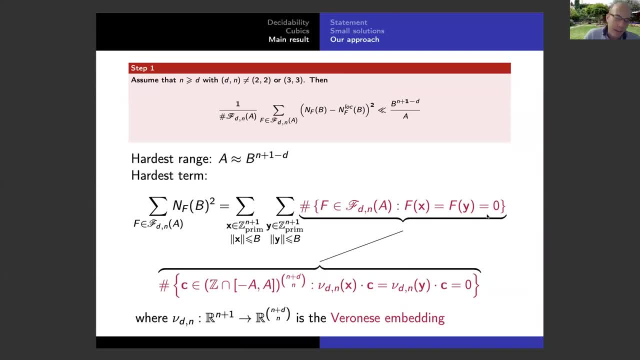 So you have this constraint that a is essentially larger than what Tim calls the hardest range here: b to the n plus one minus d. So what is the obstacle to making a smaller? We don't know how to do it. OK, That's a good one. 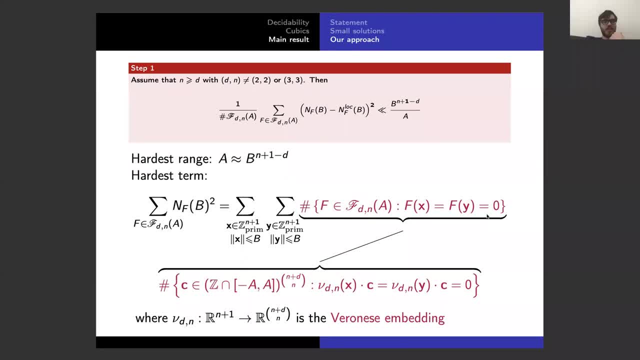 We're going to be reversing some order of summation And so then we're going to try to be getting cancellation in the sum over a. that beats some kind of trivial bound somewhere else. Yeah, And You'll probably get a flavor for it. 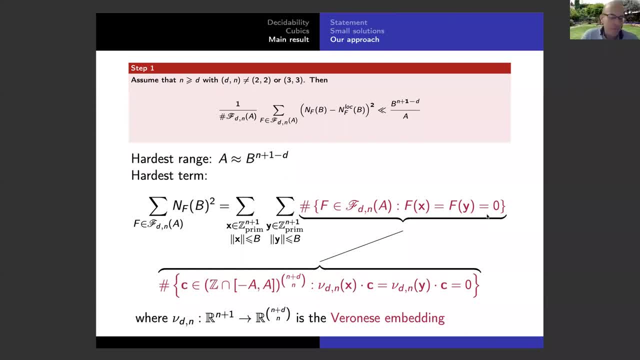 on the next slide actually, OK, OK, Thank you. Thank you for the question. So, opening up this, this second moment, and here comes the interchanging of the order of summation, as promised we, Yeah, the hardest term comes from looking at the average. 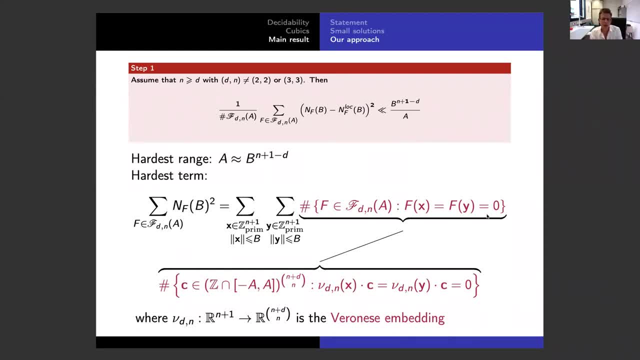 of this counting function squared, And so we open that up, and then we bring the, We interchange the order. so we're summing over now vectors x and y, primitive sine, at most b, And we're now left with counting these polynomials. 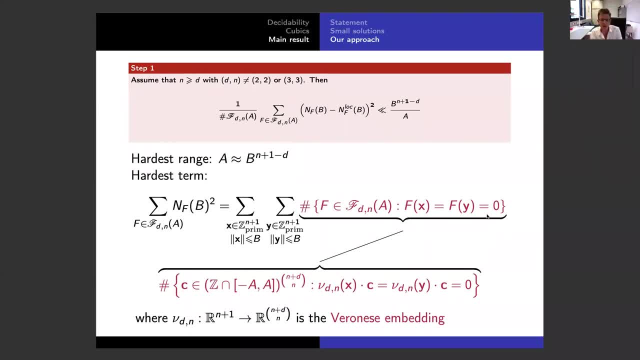 which pass through these two points. Now, that's a much easier problem. After all, what are I mean? what is the space of polynomials of degree d and n plus 1 variables? It's nothing other than a vector space of coefficients. 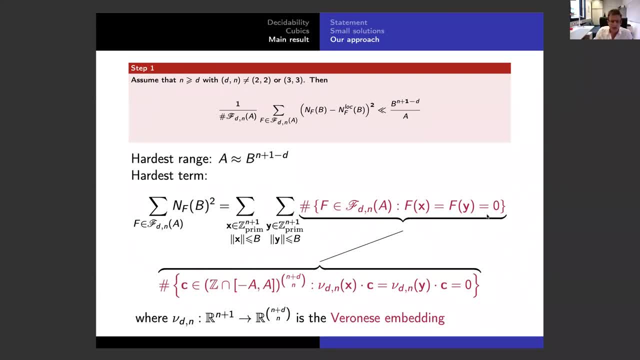 a very big vector space of coefficients. In fact, it has n choose n plus d coordinates for a polynomial, homogeneous polynomial of degree d and n plus 1 variables, And one can rewrite that problem as counting integers, integer vectors of modulus, at most a. 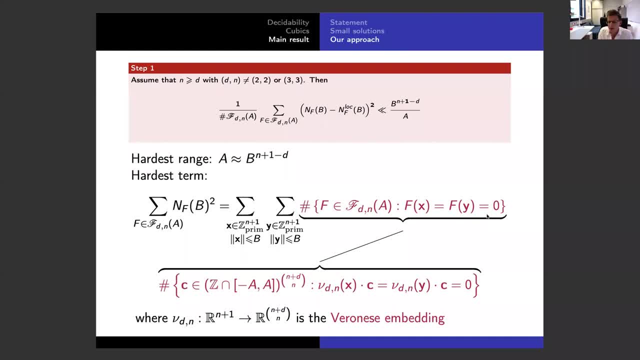 which satisfy these two linear equations. And the coefficients of the linear equations are just coming from the dth Veronese embedding of the two points, if you like, in Pn. So in principle this is much easier. We're dealing now just with 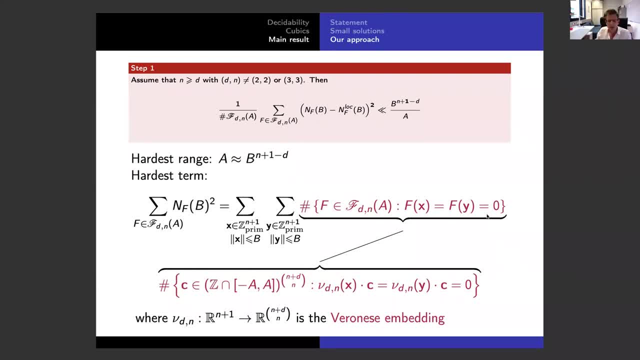 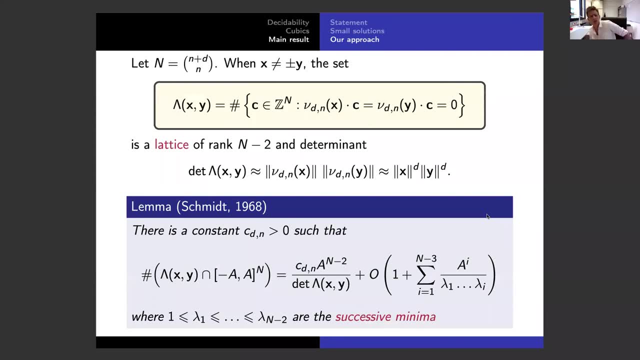 counting solutions to linear equations and in fact that's a lattice point counting problem. So let me write capital N for this binomial coefficient And, assuming that we don't have proportional vectors x and y, this set, this set of coefficient vectors, 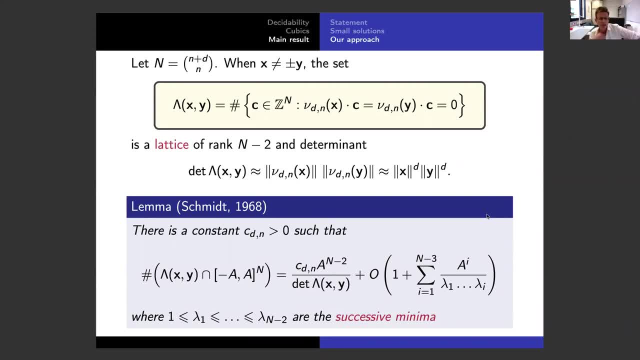 which satisfy these two linear equations, is actually a lattice And it actually has rank n minus 2.. We're cutting up two conditions And its determinant is roughly the products of the Euclidean norms of these two coefficient vectors, mu x and mu y. 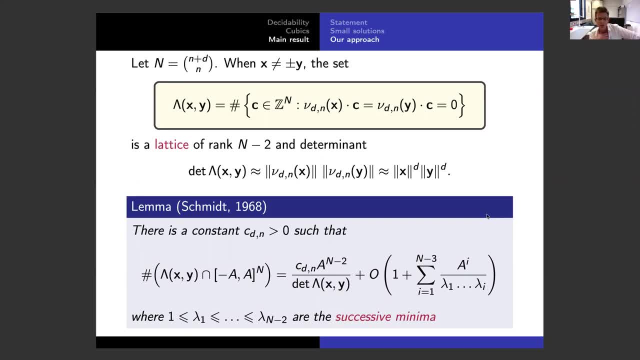 So the Veronese embedding takes you to degree d monomials. So this determinant is roughly the norm of x to the d times the norm of y to the d. So now we look up our favorite results about lattice point counting. 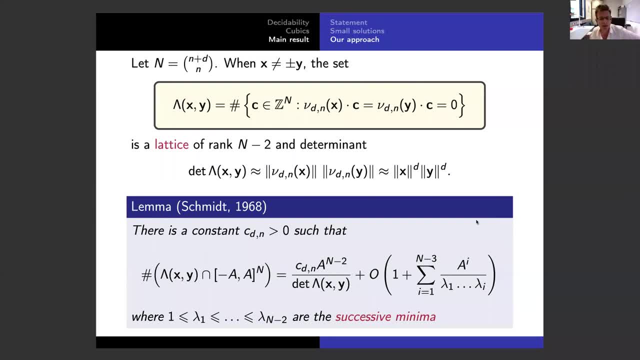 in the literature There are many. I guess I'm in Austria now, so I turn to Wolfgang Schmidt, And he tells us that the number of lattice points in this box grows like the volume a to the n, minus 2 times a constant divided by the co-volume of this lattice. 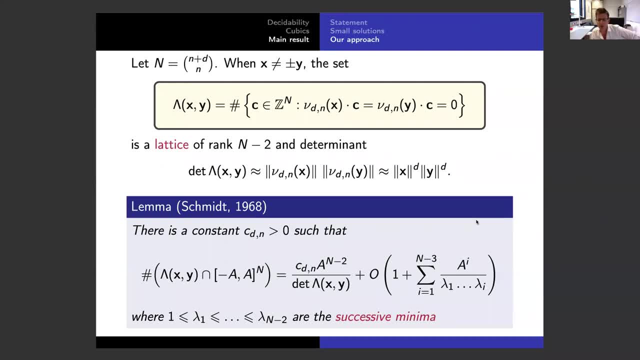 And the error term is very explicit. It's just of the shape 1 plus a sum involving smaller exponents of a and the successive minima of this lattice lambda. So remember, the k-th successive minimum of a lattice is just the minimum radius. 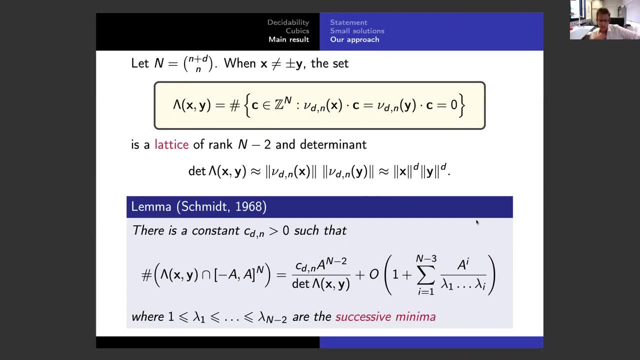 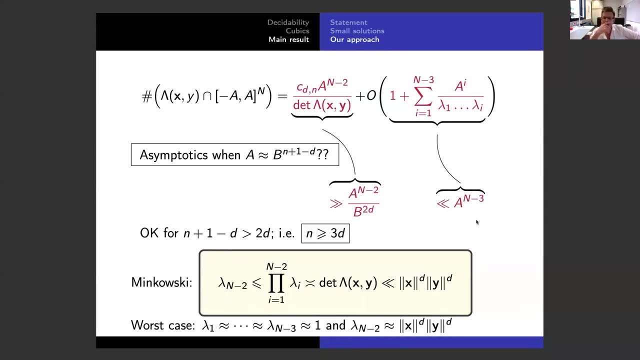 of a ball containing k linearly independent lattice points. Okay, So that's the kind of result we want to apply. I've written it again at the top of the slide. here And again we're dealing with this hard range where a is roughly. 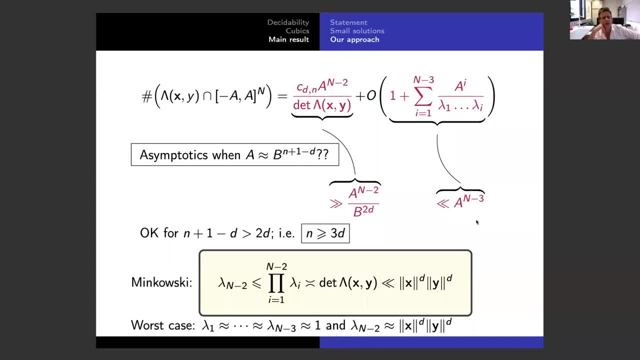 of size b to the n plus 1 minus d, So the leading term, the main term in Schmidt's result. we can see that that's bigger than a to the n minus 2 divided by the co-volume. We saw that the co-volume was like: 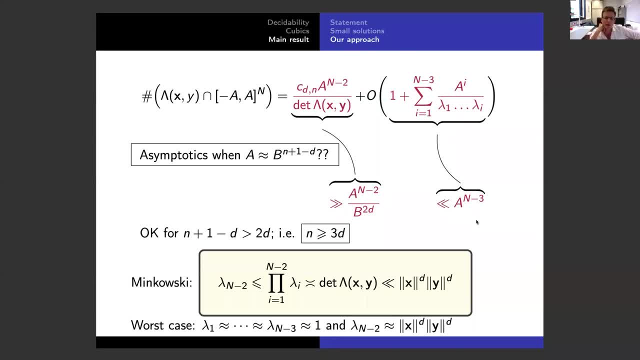 the norm of x to the d times, the norm of y to the d. x and y are both typically of size b, So the denominator there we would expect to be typically of size b to the 2d. So that's the sort of lower bound. 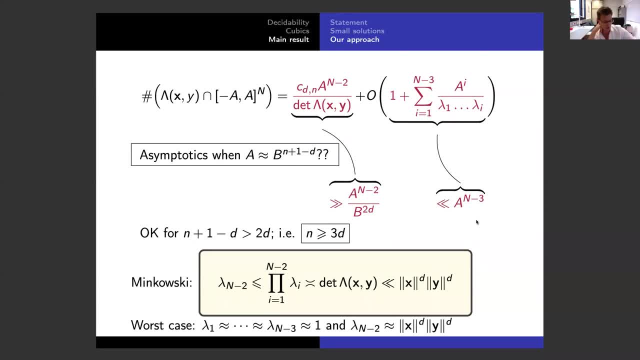 for this main term And I mean we're trying to, we're doing a sort of dispersion method, So we need asymptotic formulae for each of the terms that comes out of squaring opening up the square in the second moment. 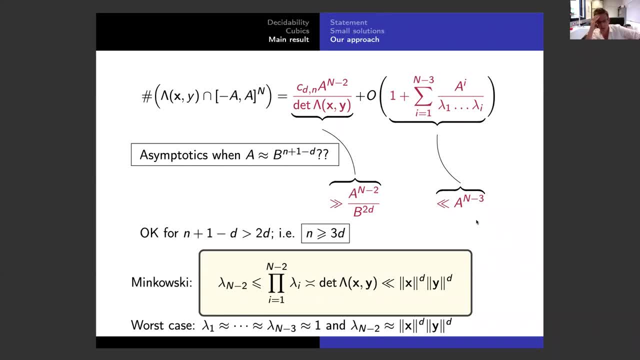 So we need to know precisely when this main term is actually bigger than the error term. Okay, So one thing we can do is observe that we are working with integer lattices, lattices which lie inside Zn, And, in particular, 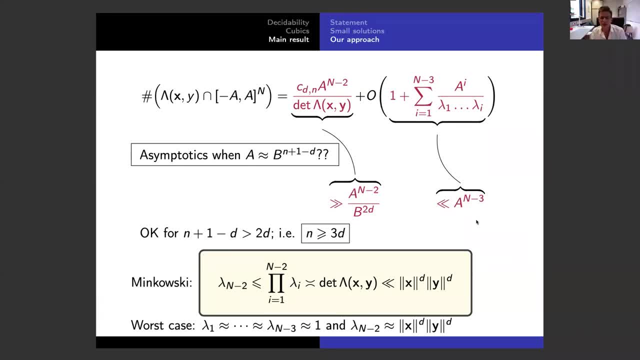 all of the vectors in the lattice are integer vectors and they all have Euclidean length at least one. So we can certainly trivially take the lower bound. lambda 1 is greater than or equal to 1, lambda 2 is greater than or equal to 1.. 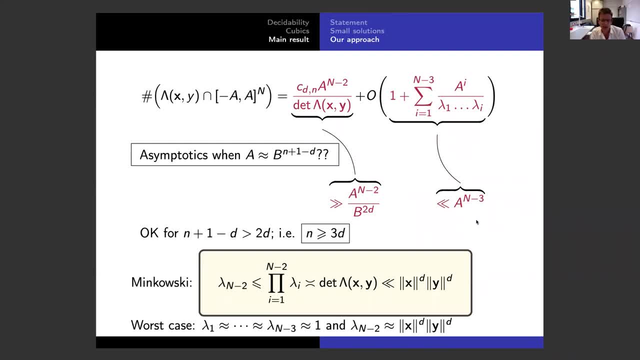 And in that way we see that this error term is bounded above by a to the n minus 3.. So if I restrict attention to this particularly awkward range where a is of size b to the n plus 1 minus d and you compare when that main term 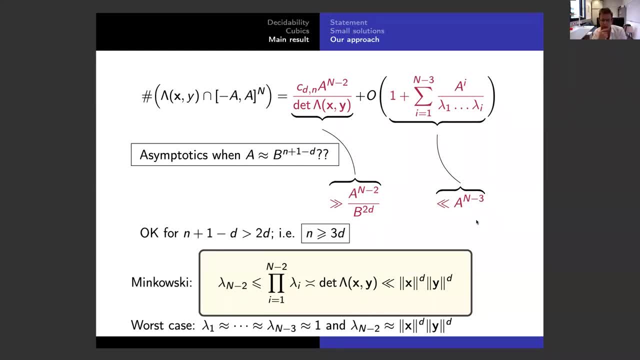 dominates the error term. you find that you need n plus 1 minus d to be bigger than 2d. So you need n to be at least 3d for this argument to work. So that's similar to the 3d. 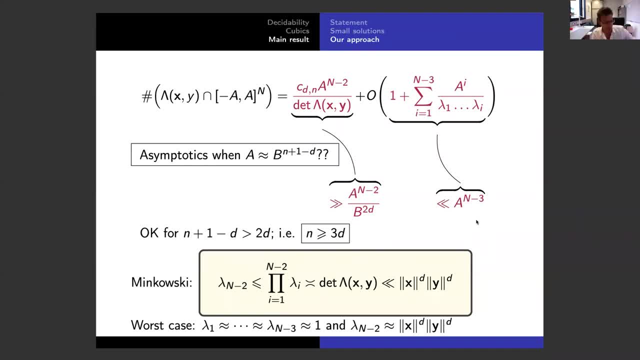 that we saw in the result by Bruden and Dietman, And I think this also shows why you can't expect to do very well unless your a is sort of sufficiently large in terms of b. Okay, well, we know rather a lot. 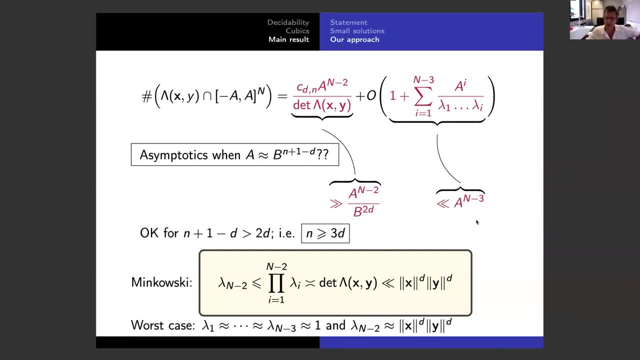 about successive minima of lattices. It's a very classical topic, So the largest successive minima is always bounded above by the product of the successive minima. The product of the successive minima by an estimate of Minkowski is bounded above and below. 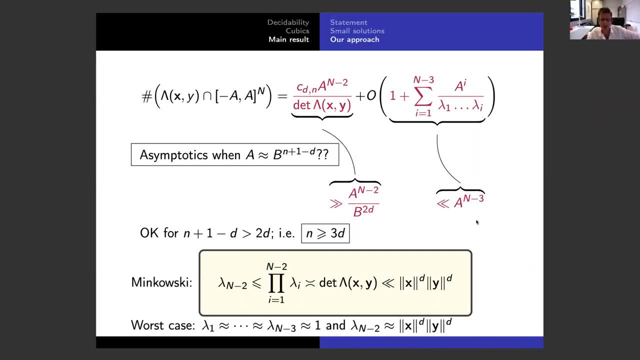 by absolute constants or constants depending on the rank, by the determinant of the lattice, and we've seen already that this determinant is roughly x to the d, y to the d. So in what I've described at the top of the slide, 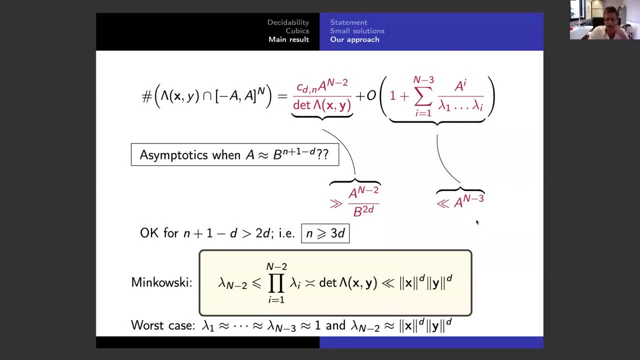 the very worst case for us is when this largest successive minima is basically the co-volume of the lattice and all of the other successive minima are one. So if we can improve that situation, if we can get better control over the largest successive minima, 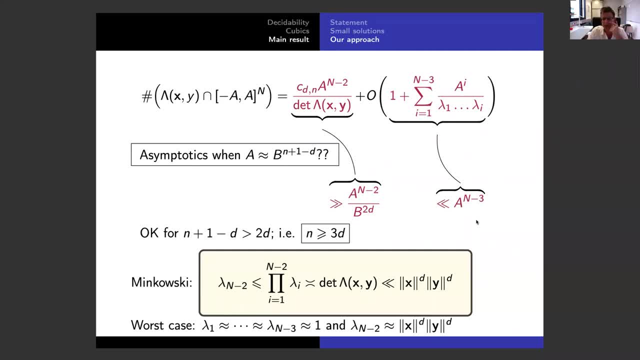 we will at Fortiori push up the size of the smallest successive minima and get, in principle, a sharper upper bound for this error term, which will allow us to handle, ultimately, a better range of n and d. So I've deliberately not left any time. 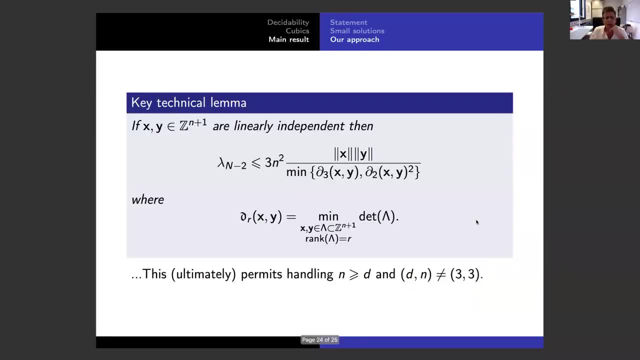 to describe the proof of the following result. but this is the sort of key technical lemma that underpins the paper essentially, and this states that provided that you're dealing with linearly independent vectors, integer vectors, then you can always bound this successive minima. 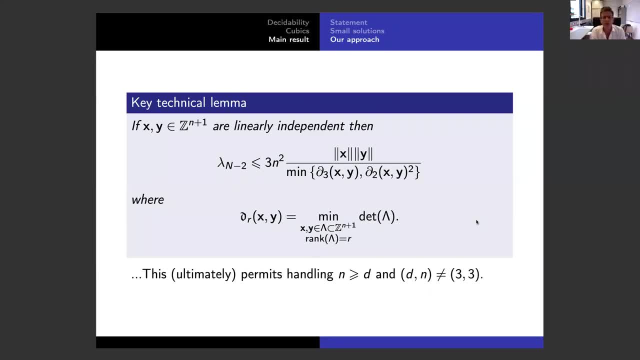 the largest successive minima, in fact all of the successive minima, by the product of the norm of x and norm of y, divided by something which is a, divided by something which it's only at least one but could in principle be larger.